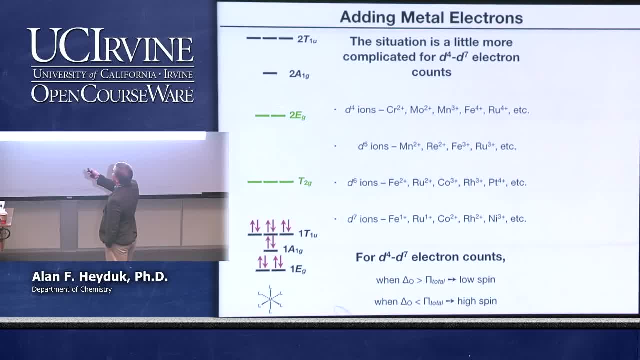 this EG, which again is the metal ligand sigma star. But these five orbitals, nominally, are the metal D orbitals. They're predominantly D in character And so they can hold various numbers of electrons. We noted that for electron counts D1 through D3, you have no choice but. 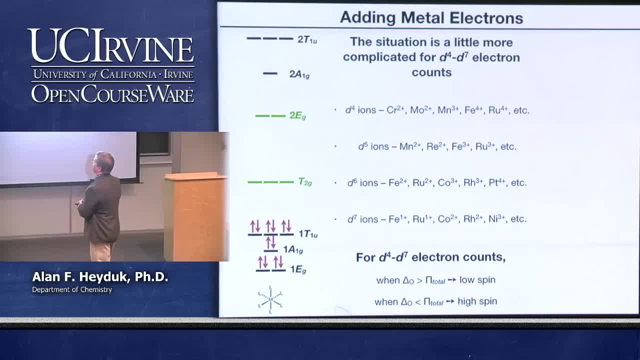 to put three electrons all spin up into the T2G orbitals For D8,, D9, and D10,. T2G is going to contain six electrons, So it's going to be a closed shell or half shell, however. 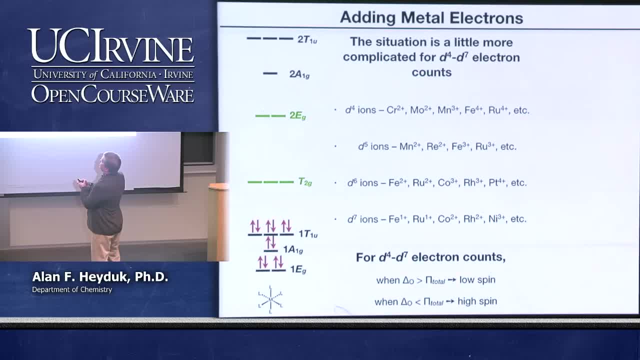 you want to think about it, And then you're going to put either two, three or four electrons up here in the EG metal ligand sigma star orbitals For D4 through D7 electron counts. you have a choice. The complex can either be high spin, which means we put in one, two. 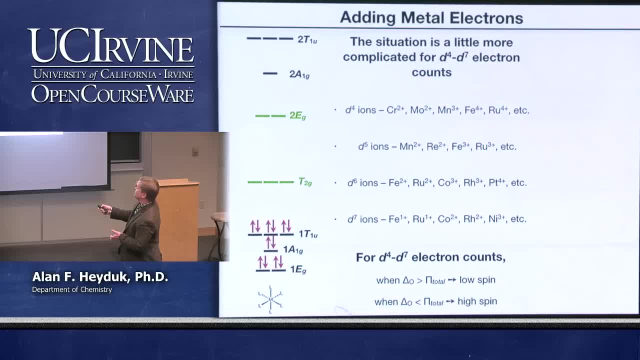 three, four goes up here, five goes here, then six, seven and eight. Or it can be low spin, where we put electrons: one, two, three and then four goes here, five goes here and six goes there, followed by seven and eight. Now the difference between a high 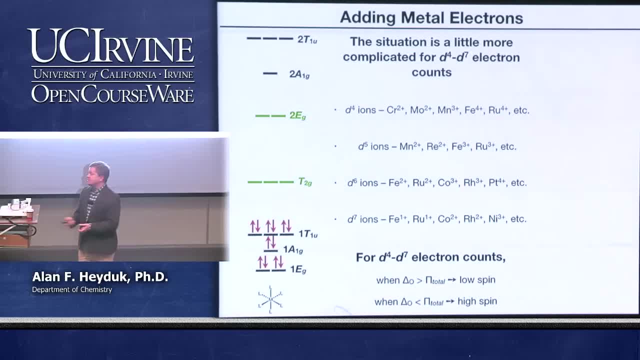 spin and a low spin complex really comes down to the difference between this energy gap and the electron pairing. energy Electrons are negatively charged. Putting two negatively charged particles in the same orbital results in a repulsive interaction, because negative charges repel each other. 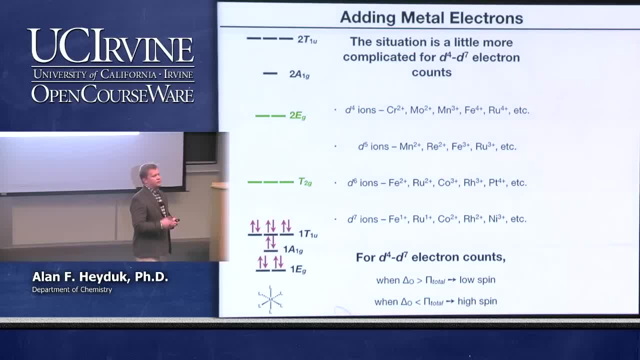 A point that I will try and remember to emphasize over and over and over again. This question of high spin versus low spin really only applies for our purposes. it only applies for octane dihedral complexes. Moreover, it only applies to metals in the first row of the transition. 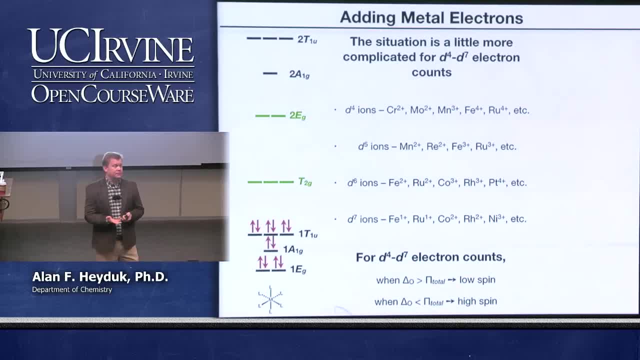 metal series, So three D metals, The metals in the second row of the transition metal series, the metals in the third row of the transition metal series, are always low spin. Similarly, and we'll see why in a few minutes, tetrahedral complexes of the three D metals. 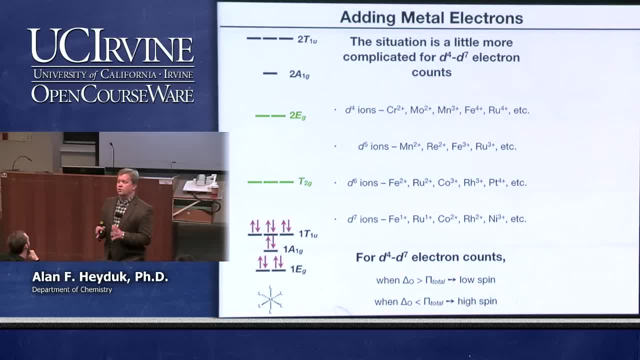 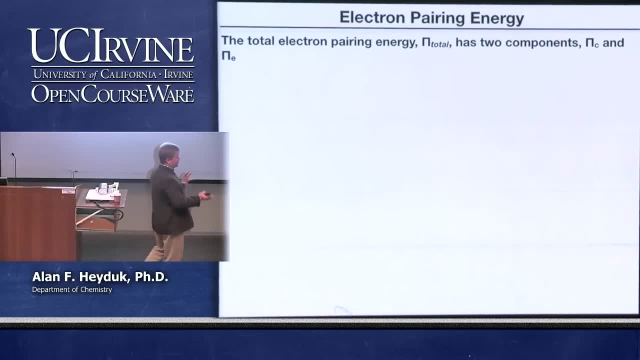 of that first row are always high spin. Okay, and we'll come back to that, But I want to talk about how we compare electron pairing energy and delta O, the splitting between the T2G and the EG orbitals. And so when we talk about the total electron pairing energy, there's two components. What? 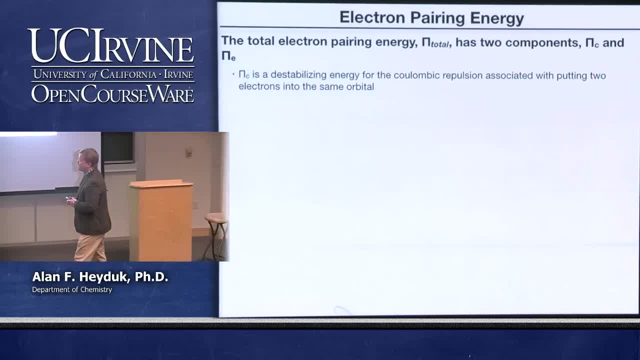 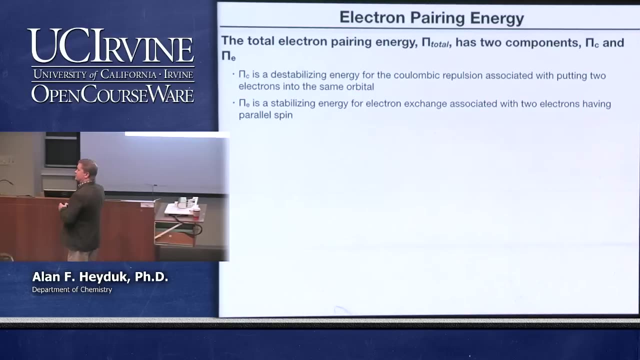 we can call pi C and pi E. So pi C is a coulombic term. It's what I was just telling you. Two negative charges are going to repel each other. when you try and put them in the same small region of space, It turns out that there's also a stabilizing influence of pairing up. 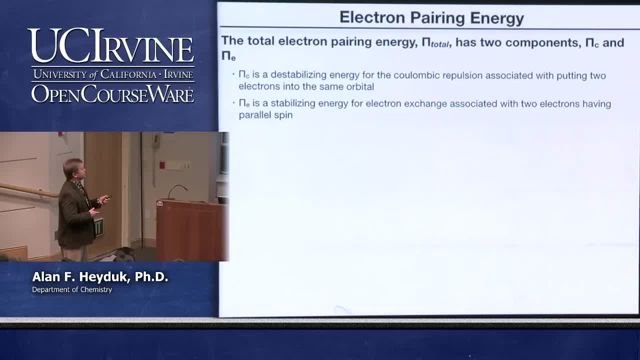 electrons Pay that data, okay, and go over it another couple of times, okay. Well, this is one of these funky quantum mechanical things. Okay, If you have two electrons with the same spin, you get a stabilizing effect that we call exchange, because basically you can't tell. 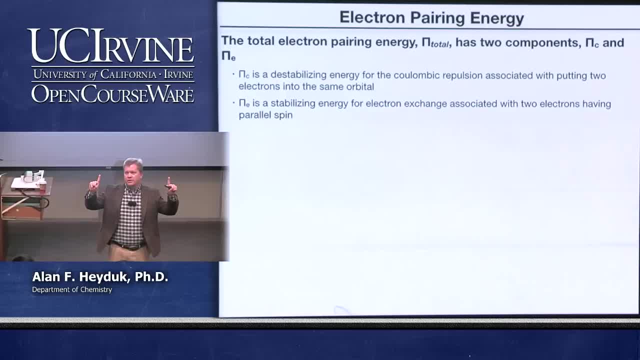 one electron from another, And so it's a stabilizing energy. when you can do this versus this, okay, when the electron is on one position versus when it's on the opposite. If that's the case, then you simply want to call that transition When the electron is on one position or without gutter reaction. this would be going to give you a chance to get goingお. 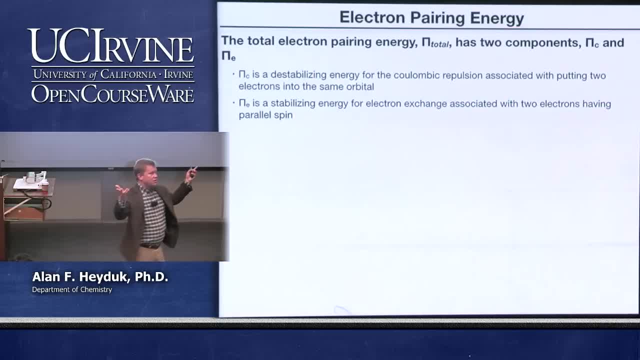 the electrons have the same spin. you can't tell them apart, so you can't tell that Fred is going to be on the left and Barney's going to be on the right. okay, they're indistinguishable. now, what is this? what is that really? it's actually. 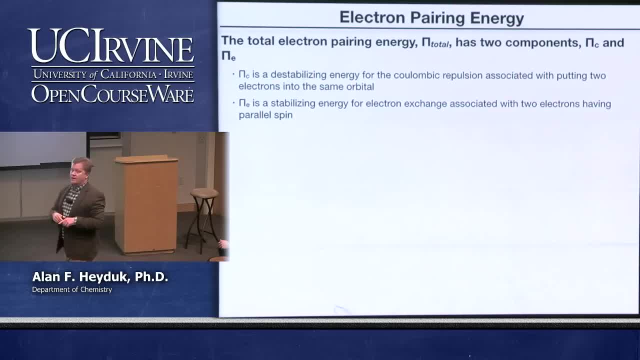 kind of an entropy thing, right, if you have two spins, two electrons at the same spin, this is degenerate with this, so you have more microstates and it's a lower energy configuration. so if we consider the d4 case, high spin, the total pairing energy, we're going to have three exchange components and zero coulombic. 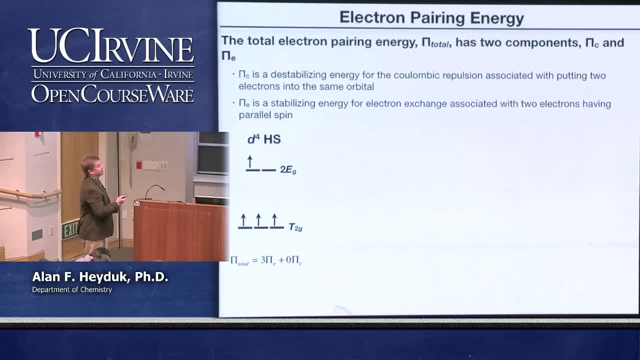 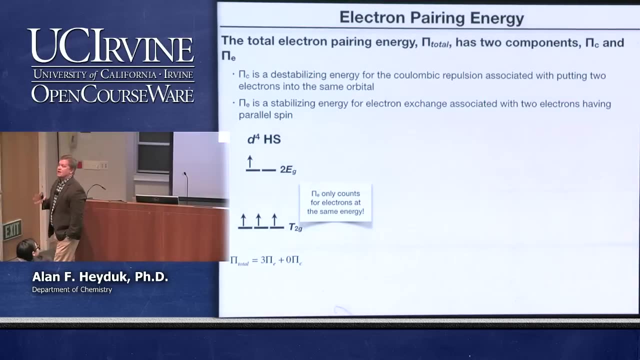 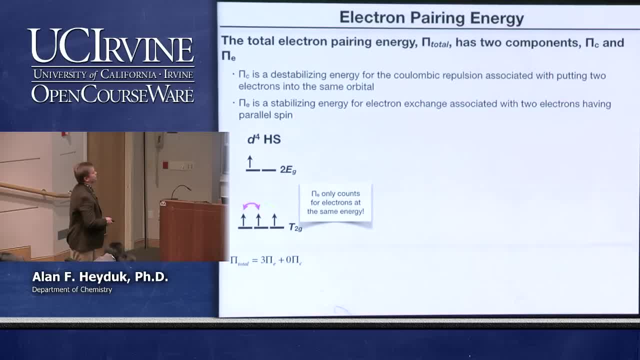 and, and, and, and, and get an exchange component for this middle electron and the right electron and you get an exchange component between the left and right. so there's three different ways you can swap electrons. so you get three of these exchange components: right, right, change stabilizations. 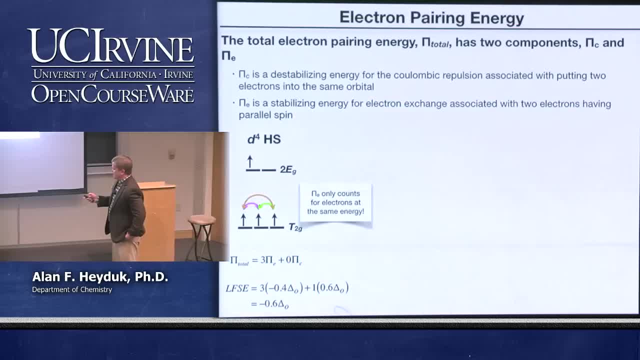 It's important to note that it only happens when the electrons are in orbitals of the same energy. So remember we said that a T state is a triply degenerate. representation Part means all three parts are identical, indistinguishable: same energy. 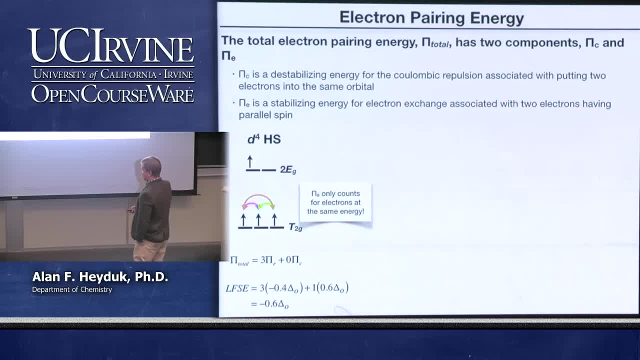 In this case we can also calculate the ligand field stabilization energy. We calculate it the same way we calculate the crystal field stabilization energy. We have three electrons in the T2G. We multiply that by minus .4 delta O, We have one electron. 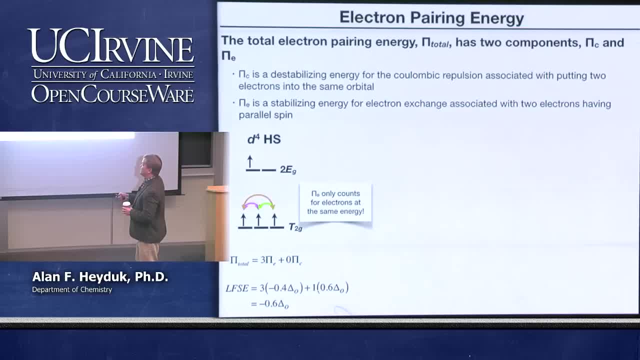 In eG that's multiplied by positive .6 delta O, and so when we're trying to make a decision whether this going to be a high spin or low spin case, we have to consider the total pairing energy and this ligand field stabilization energy. 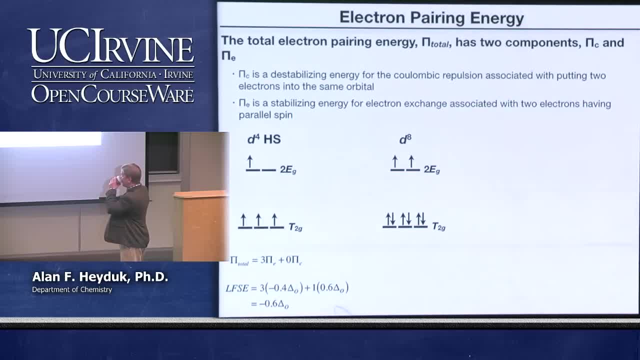 Gratuitous use of animation. I know it's great In the D8 case. Here we have a lot going on for the pairing energy. Obviously we have three orbitals that are doubly occupied, so we're gonna have three contributions from coulombic repulsion. 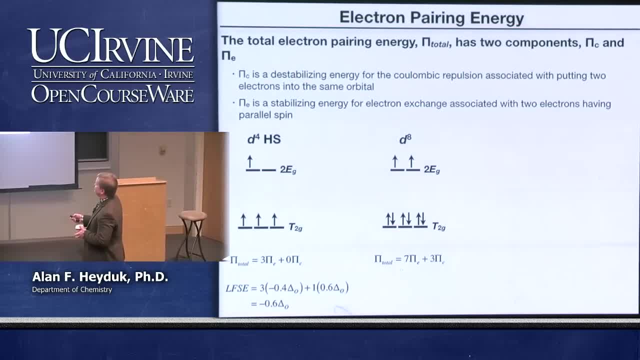 We have seven exchange components. It's easy to see you have one here, but it turns out that you also have six down in the T2G For the spin up on the left, spin up in the middle, spin up in the middle to spin up on the right and then spin up on the left to spin up on the right. 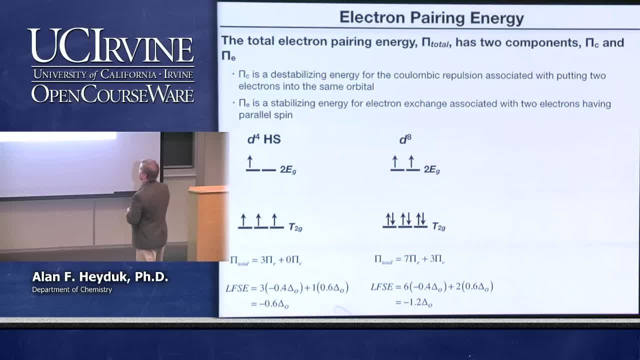 There's three. and then the spin downs also contribute an exchange component. The ligand field stabilization energy is negative in this case because we're putting most of the electrons in the T2G. Okay, D6, low spin, everything goes into T2G and if you were to calculate the pairing energy, 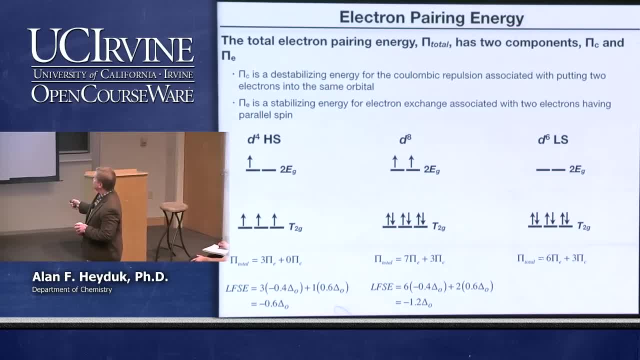 we have six exchange terms, three coulombic terms and the ligand field, stabilization, energy is everything is in the T2G. Yeah, There's only one right, Because there's only one way to swap. Okay, So you know, taking the left and putting it on the right is the same as. 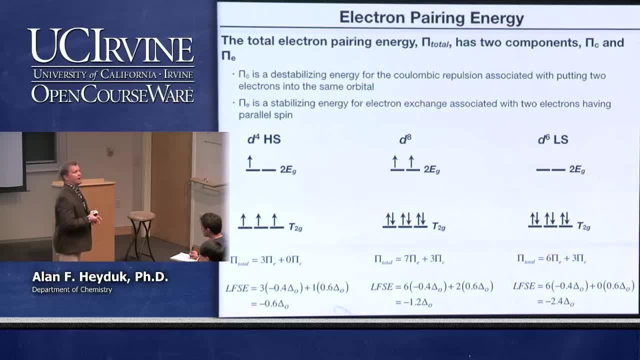 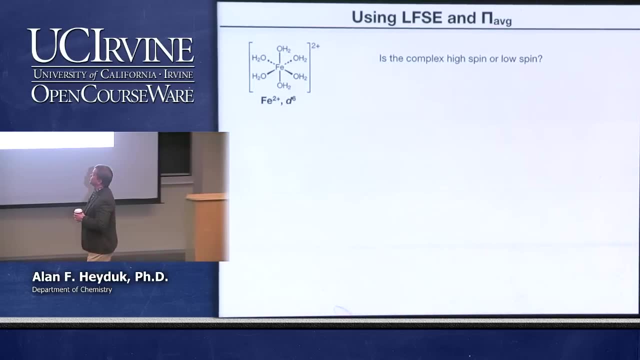 taking the right and putting it on the left. So there's only one swap possible. So you only get one exchange: energy. Any other questions? All right, So we can consider something like a D6 hexaqua iron. Ask if it's going to be high spin or low spin. You can go in the back of your textbook. 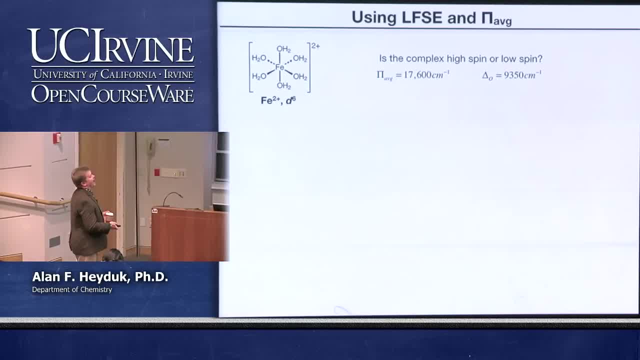 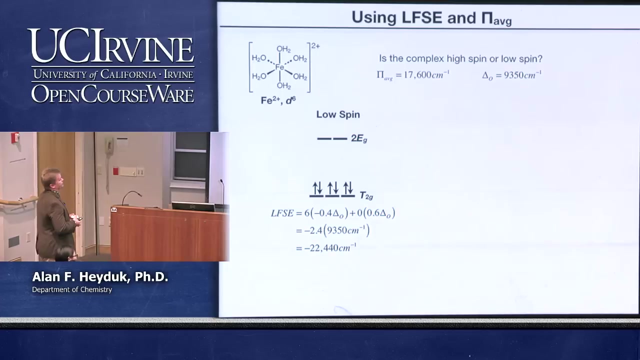 or you can Google search it There's. people have tabulated average pairing energies. Delta O is known for iron in the 2 plus oxidation state. With six water ligands around it We can calculate what the low spin ligand field stabilization energy would be. 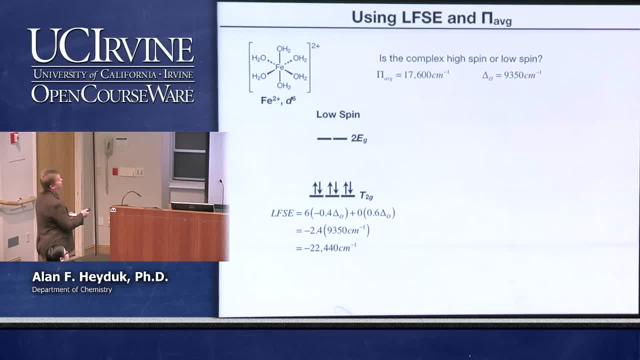 If we put all six electrons in T2G we're going to have six times minus point four delta O. So that's going to give us a ligand field stabilization energy of negative 22,440 reciprocal centimeters. The total energy in this case is going to be three times this average. 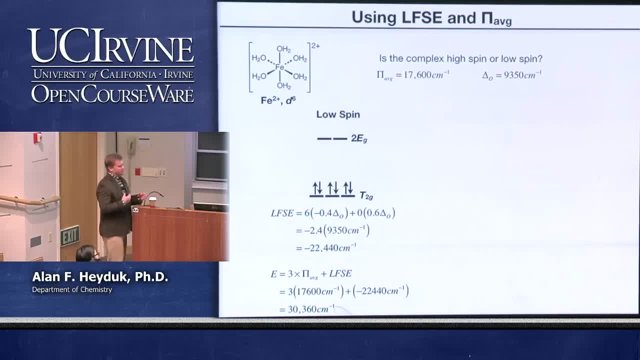 pairing energy. Okay, So this pi average already includes exchange components and coulombic components, So three times 17,600 wave numbers. we add in the ligand field stabilization energy and we calculate that the energy of this low spin state is 30,, roughly 30,000 wave numbers. 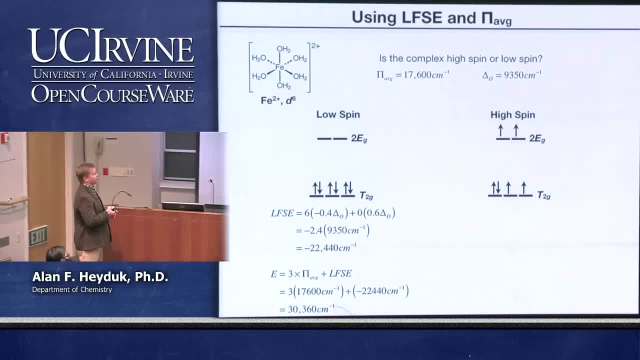 We can compare that to the high spin electron configuration. assuming the same delta O value. assuming the same pairing average pairing energy, We calculate a much less negative ligand field stabilization energy. But of course we also have one pairing going on. 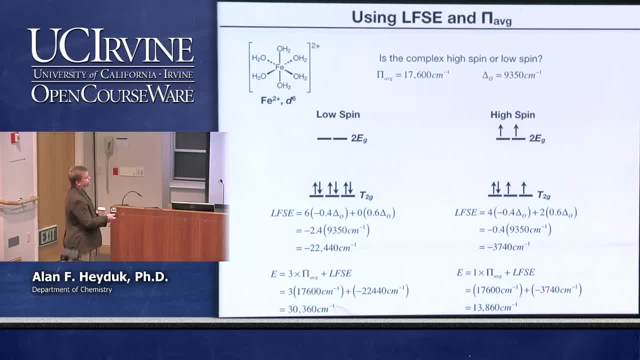 And so we calculate overall that the energy is lower. Lower energy species are the more stable species, and so, in this case, iron two with six water ligands is indeed going to be a high spin configuration, because it minimizes the overall energy. That minimizing of the overall energy comes about because of this reduced 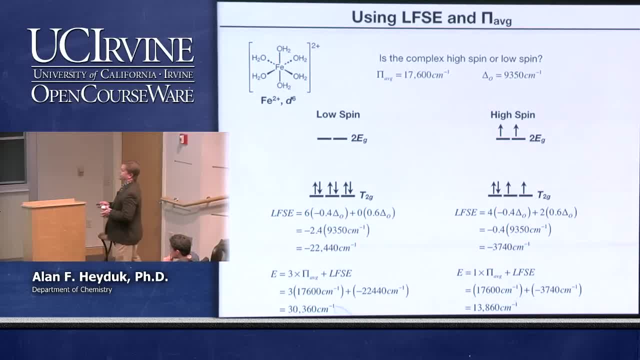 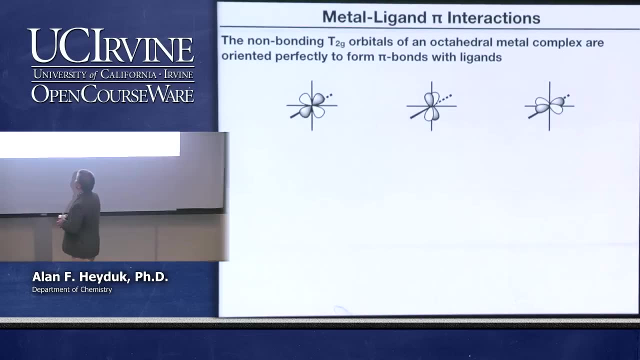 pairing energy, not because of a reduced ligand field stabilization. Based on ligand field stabilization, we'd expect low spin to be favored, but it isn't Okay. So at this point everything seems straightforward. Alright, calculating the bonding manifold for an octahedral complex seems pretty easy. 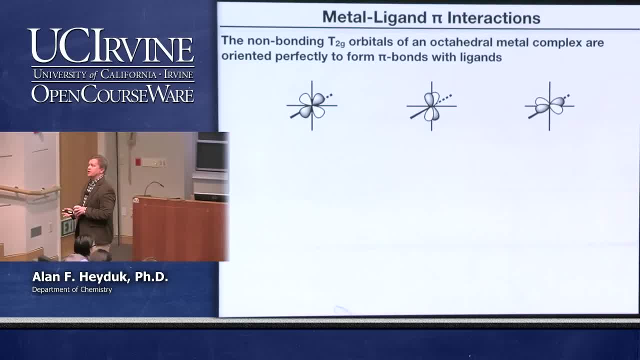 But at this point all we've concerned ourselves with is sigma bonding, The donation of a single lone pair of electrons from the ligand, the Lewis base, to the metal, the Lewis acid. That left us with a T2G Okay. 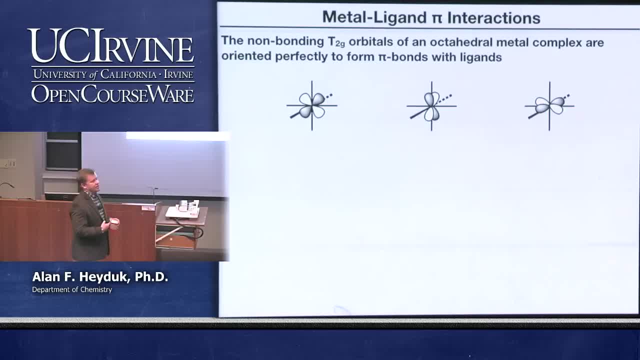 G orbital set, the XZ, the YZ and the XY- orbitals that we said were non-bonding in an octahedral metal complex. That's only true if you have ligands that are strictly sigma only. Okay, They only have a lone pair of electrons to donate. 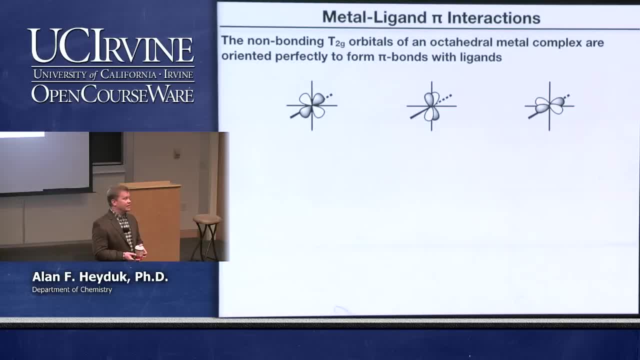 Okay, A perfectly good example of a sigma only ligand is ammonia. Okay, The nitrogen has one lone pair that it can donate to the metal. All of nitrogen's other electrons and orbitals are tied up, making NH bonds. Okay, So it can only act. 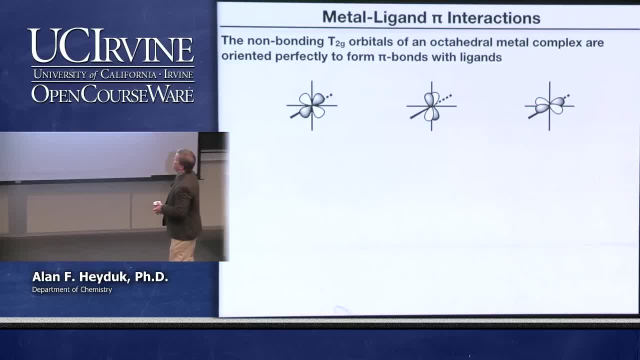 as a Lewis base, donating two electrons to the metal. But if we look at this right, I don't think it's too big of a stretch to look at these orbitals and say, huh, I'll bet you if you had a ligand right there. 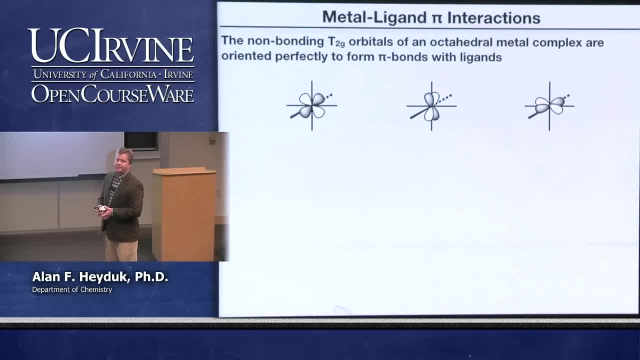 with a P orbital on it, you could make a pi bond. In fact you could kind of convince yourself that you're making four pi bonds with that single D orbital. Now it turns out you don't. one D orbital cannot make four pi bonds. 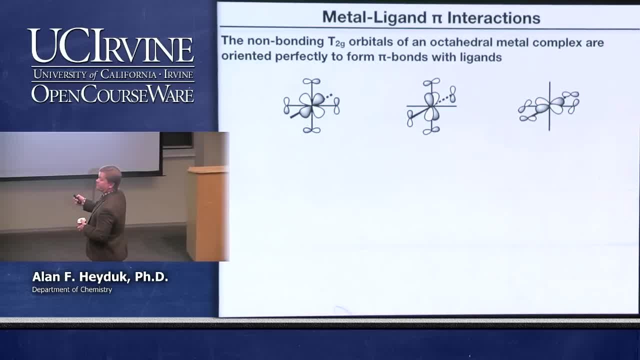 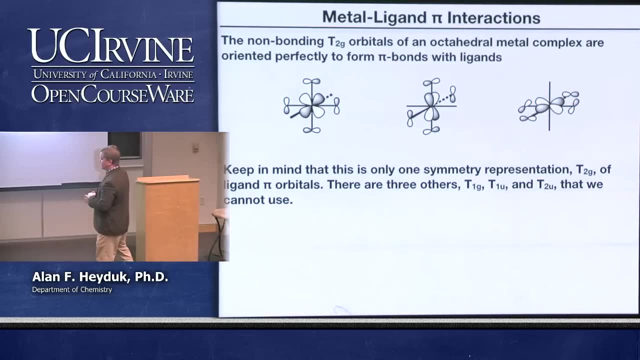 It can make one pi bond delocalized over four different ligands- Okay, But it can't make four bonds And we can do this for all three. We can do this for all three of the T2G-like orbitals. Now, what kind of a ligand might be able to participate? 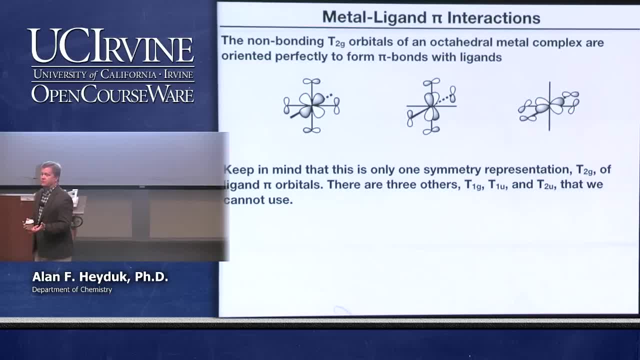 in this kind of bond, this pi bonding with the metal. Well, how about something simple like a chloride, right Where it's, where we know chloride is going to have a lone pair that it donates to the metal to make the sigma bond? 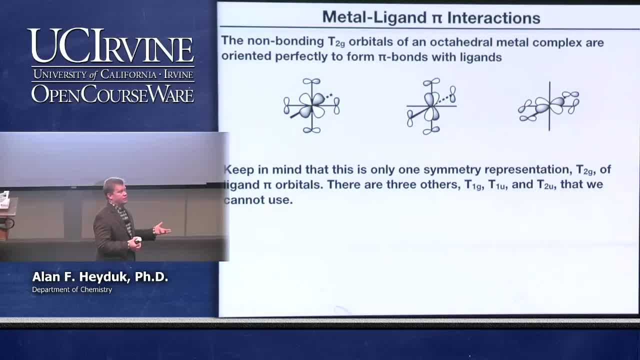 But then if we did a Lewis base we'd have a P bond. But then if we did a Lewis dot structure for chloride we'd still put three lone pairs, And we know those lone. some of those lone pairs would be in orbitals that look like that or like that. 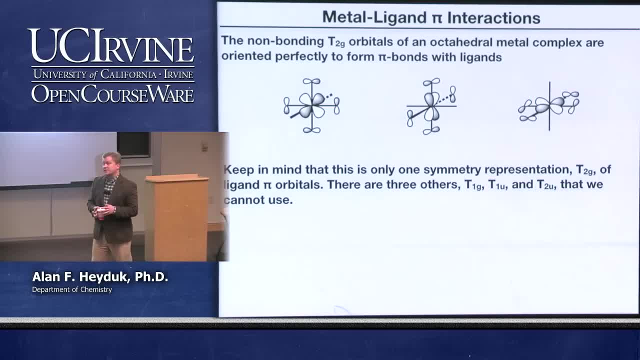 It turns out, if you were to have something like tungsten hexachloride, each one of the six chlorides would have two pi symmetry orbitals that could donate to the metal. You go through and figure it out Right: Six ligands times two pi orbitals on each one is 12 possible pi. 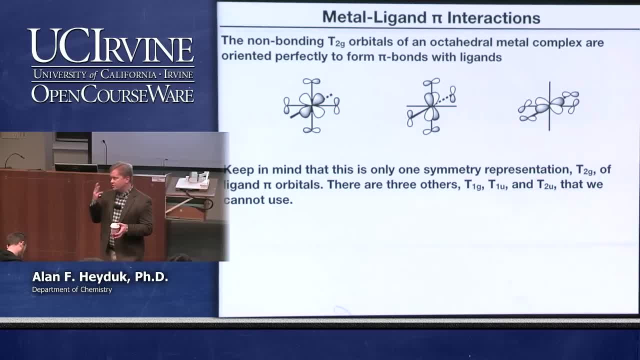 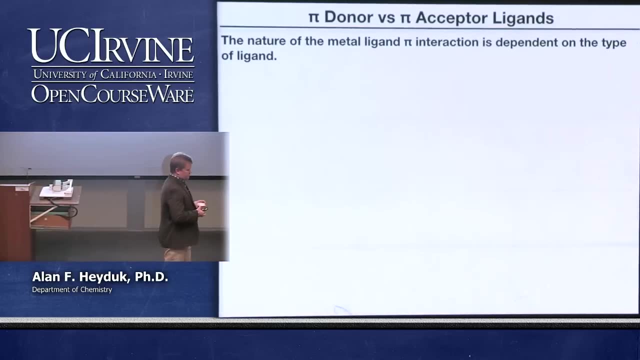 donations, but only three of those are of the proper symmetry to interact with the metal T2G- It's the ones shown here- Becomes one of these really hard projection operator problems. So we just said that a ligand- ligand like chloride or a bromide, something with lone pairs- 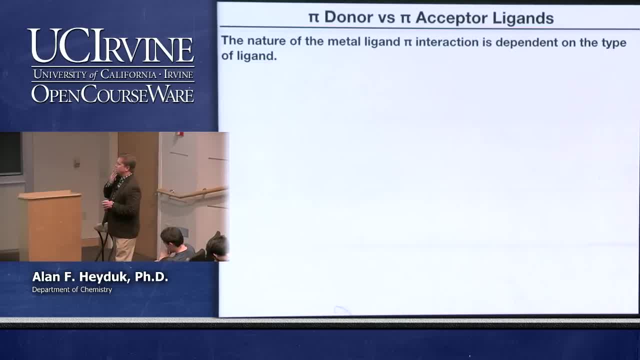 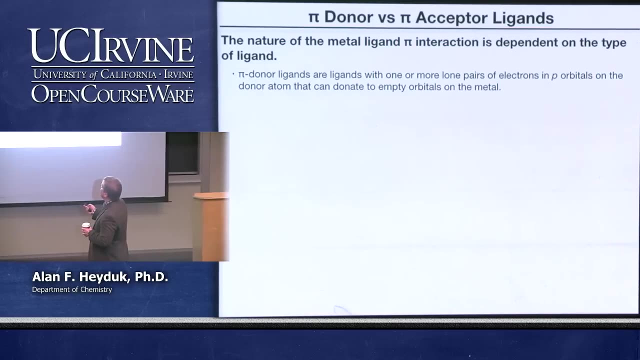 of electrons can probably participate in pi bonding with the metal. Turns out that those aren't the only cases, And this is another place where transition metals complexes- can be pretty special. So something like a chloride or a bromide is what we call a pi donor ligand. 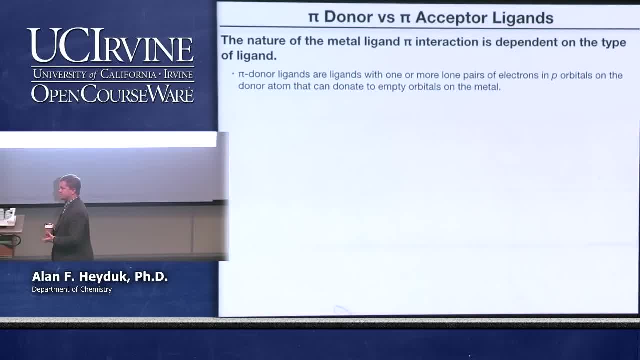 And so we name it a pi donor because it's got lone pairs of electrons in orbitals of pi symmetry with respect to the metal ligand bond. So you can think about it: as chloride can act as a double Lewis base, It donates the first pair of electrons to make the sigma bond. 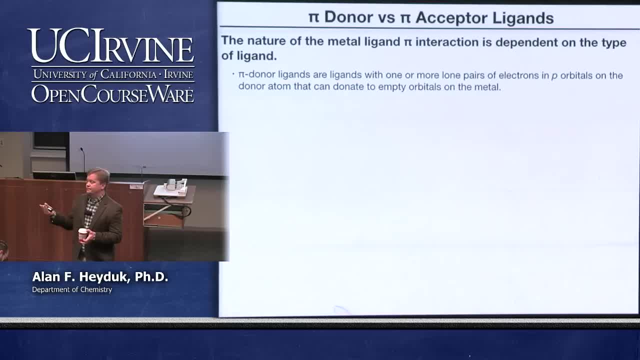 And then it can donate a second pair of electrons to make a pi bond. So if we're just looking at one of these, there's your metal d orbital that's empty. There's your chloride p orbital that has a pair of electrons, And we donate the electron density. 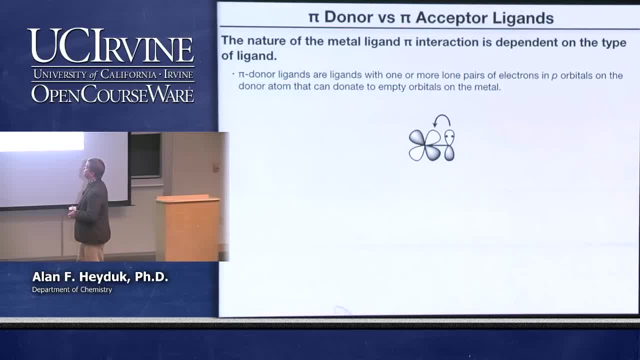 to make the metal ligand pi bond. There's a whole host of examples And if you look at this list, it's generally heteroatom type ligands. right? There's your halogens, alkoxides, thiolates, azonidose, oxidose, imidose, nitridose. 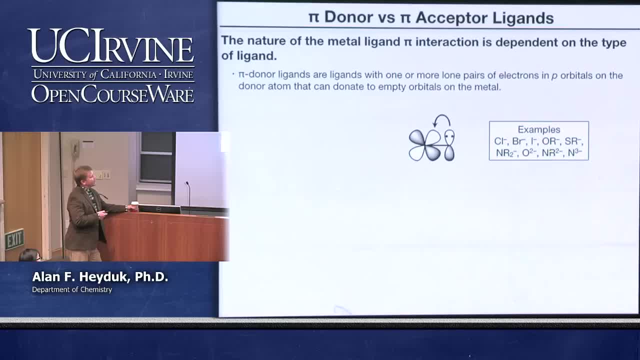 All these things with heteroatoms negative charges. We would put lone pairs on them If we did full Lewis structures. they can all donate an extra pair or two of electrons to an empty metal orbital. But there's a whole other class of ligands that can pi. 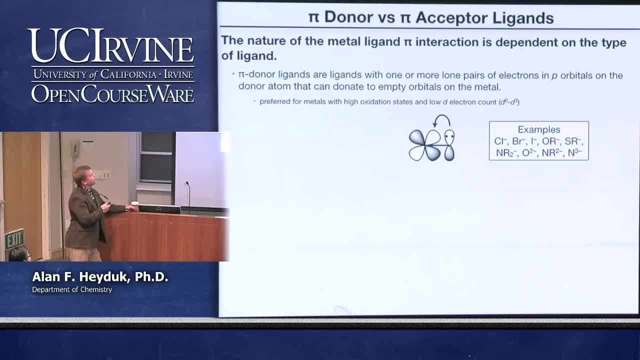 Oh, okay, sorry. This type of bonding is preferred with metals with high oxidation states and low d electron counts- D0 through D3 at the most. Why? Why would this kind of an interaction be favored for very low d electron counts? 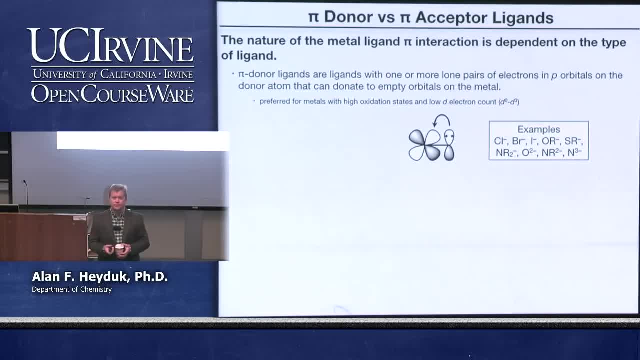 Hmm, A lot of open orbitals, right? What we're effectively describing here is another Lewis acid Lewis base type interaction. The ligand, now, in a pi sense, is acting as a Lewis base towards the pi Lewis acid of the metal. Well, that means the metal orbital has to be empty, right? 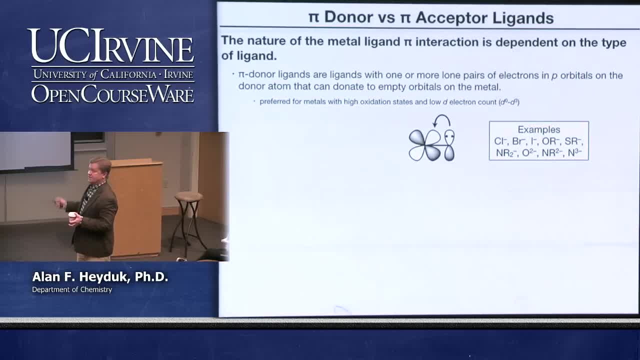 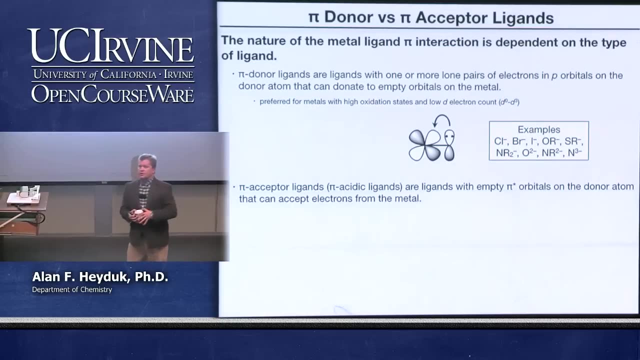 The metal. that orbital is not going to be acidic if it's got electrons in it already. The only way for T2G orbitals to be empty is if you have very low electron counts. So there's a whole different class of ligands. 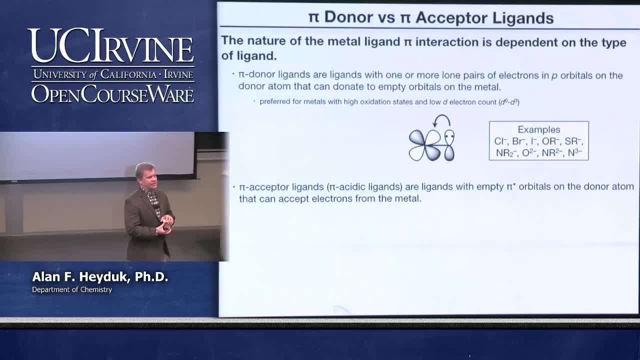 that can participate in pi bonding and they're called the pi acceptor ligands. So we literally turn the idea on its head. these ligands will also often be called pi acid ligands because in our Lewis acid- Lewis base paradigm the ligand acts as a pi Lewis acid. 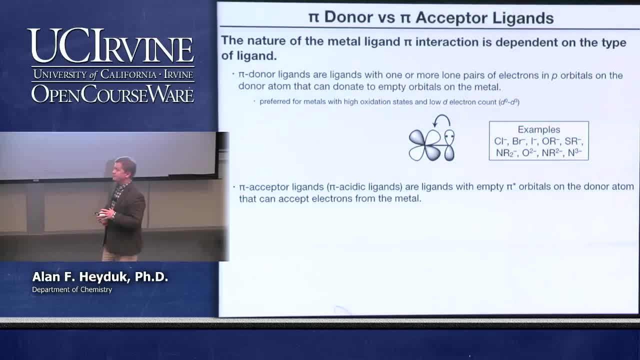 It accepts electrons back from the metal, And so the prototypical example here is carbon monoxide: The homo, or sorry, the lumo of carbon monoxide. the lowest unoccupied molecular orbital is a pi star orbital. It's localized on carbon and it's empty right. 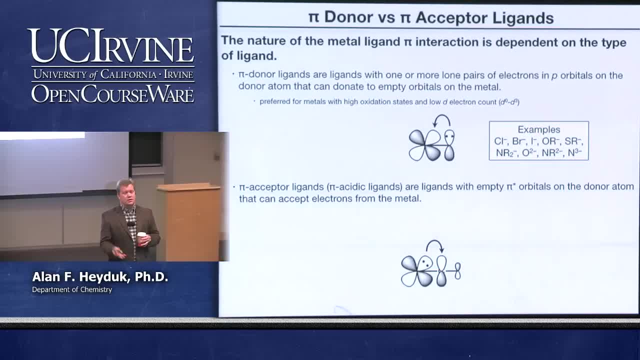 This is, carbon monoxide has a triple bond. The pi orbitals are filled, It has a lone pair on carbon that it can donate to the metal to make a sigma bond. And then there's a low energy orbital, a pi star orbital. that's empty. 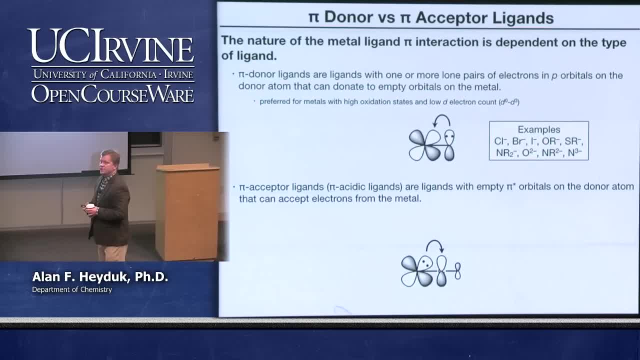 And so if the metal has a pair of electrons in this T2G orbital, it can donate backwards. This is still a pi interaction between the metal and this carbon right. It's just the electrons are still there, So it's empty. 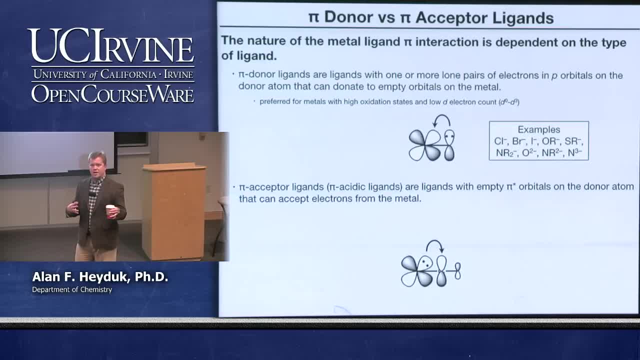 The electrons are starting on the other fragment. We're not used to thinking about the electrons, about the metal being the Lewis base, but here it is In a pi sense. the metal is Lewis basic and the CO ligand is Lewis acidic in the pi manifold. 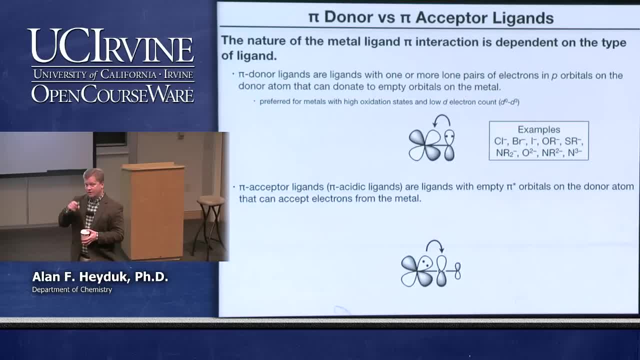 CO is still a Lewis base. in the sigma donation It donates a lone pair from carbon to the metal to make this sigma bond but then the metal gives back some electron density through the pi bond. It's a synergistic. You can think about it as being a synergistic effect. 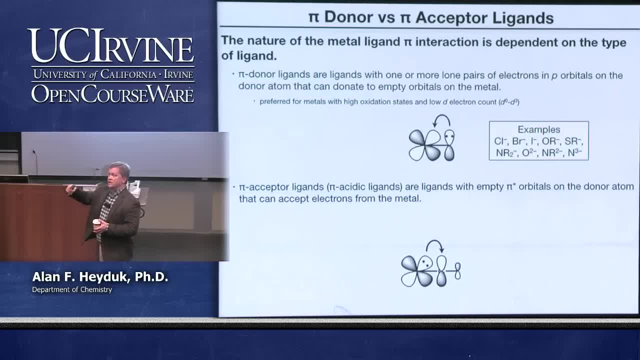 The more sigma donation the carbonyl is, the easier it will be for the metal to give back some electron density through the pi bond. Carbon monoxide, nitrogen monoxide, pyridine olefins are all examples of ligands that can act as pi acceptors. 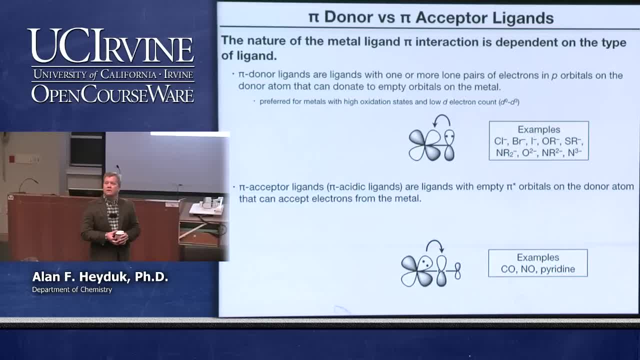 Yeah, The lines across the center of the ovals are those representing sigma bonds. Yes, for right now that's representing the sigma bond. So we're assuming that, And then we're assuming that, And then we're assuming that. 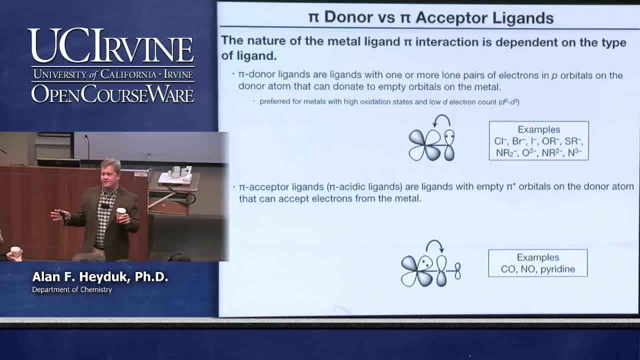 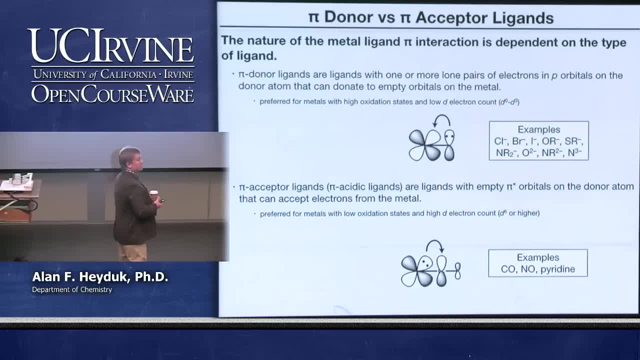 Okay, Now, obviously, if this interaction requires the metal to donate electron density back to the ligand, then you're going to need metals that have a high electron count. T2G is going to have to have electrons, And so typically these are metals in low oxidation states. 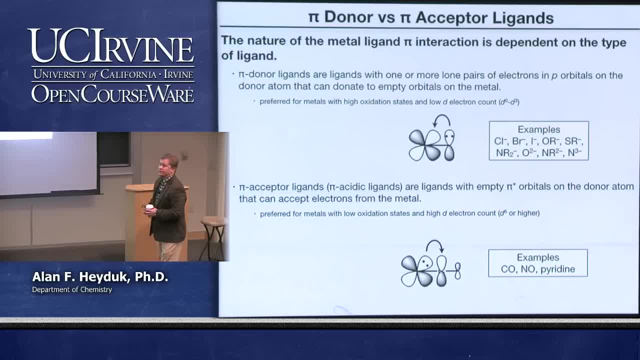 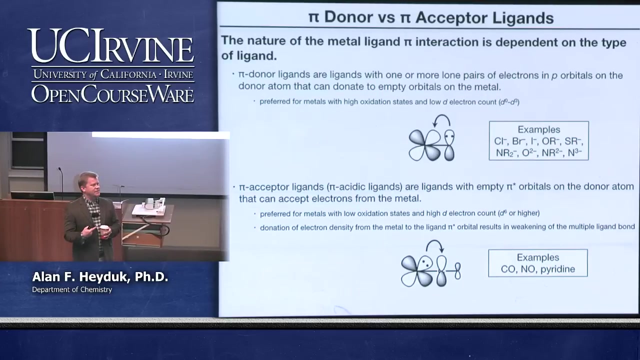 with high D electron counts, six or higher, Especially in a low spin configuration. Now some of you that are thinking a step ahead are probably asking yourself: Well, wait a second. What happens if we donate electron density into a CO pi star orbital? 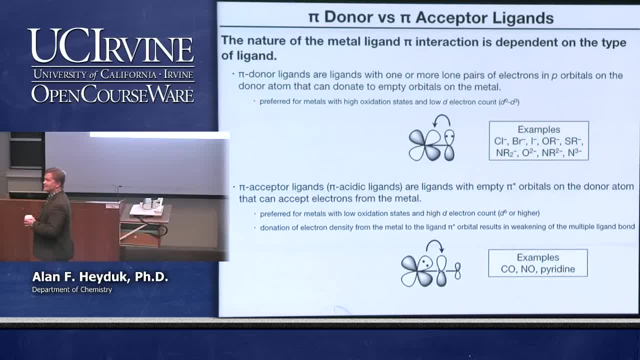 We know that if we start populating an anti-bonding orbital, it weakens the bond Right, And that's exactly what we see for carbon monoxide complexes of transition metals. Free carbon monoxide has a triple bond between carbon and oxygen. 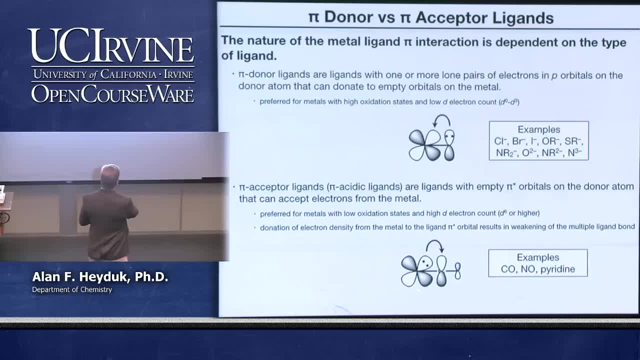 When we bind it to a bond it's a triple bond. When we bind it to a transition metal, we get this back. donation of metal electron density into the carbon oxygen pi star And the CO bond distance expands The CO vibrational frequency that we measure. 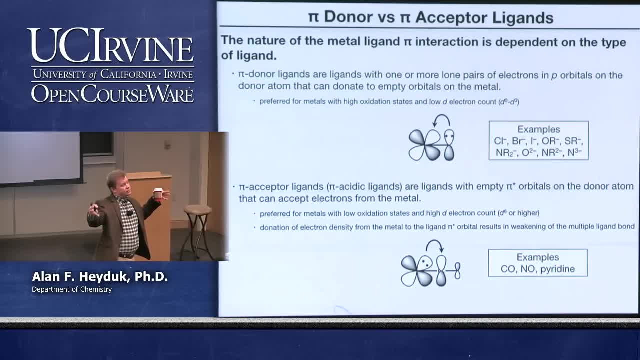 in the IR gets indicates a weaker bond. Okay, So everything the picture holds together That the metal's acting as a Lewis base, donating into an empty pi star orbital on the carbonyl and weakening that carbon oxygen triple bond. 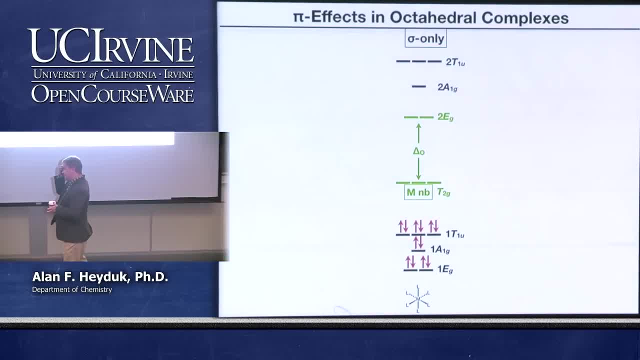 Okay. So let's go back to our old friend, the octahedral molecular orbital diagram. This is just what we derived on Wednesday. I'll remind you again. Here are the. Here are the six metal ligand sigma bonds. Okay, That's the sigma bond where the ligand is acting. 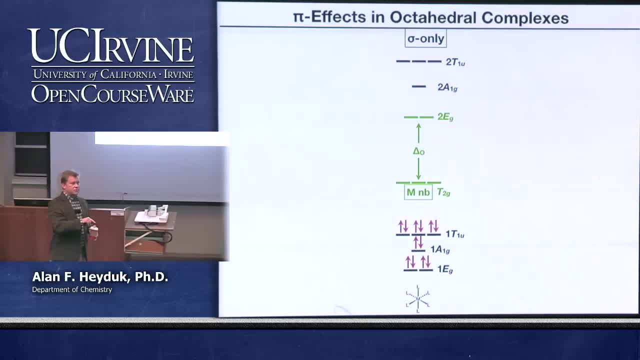 as a donor to the metal. These are always going to be here. Okay, Represents the Lewis basic ligand donating two electrons to the metal to make the sigma bond. We have our anti-bonding orbitals up there And in the middle right we have our five d orbitals. 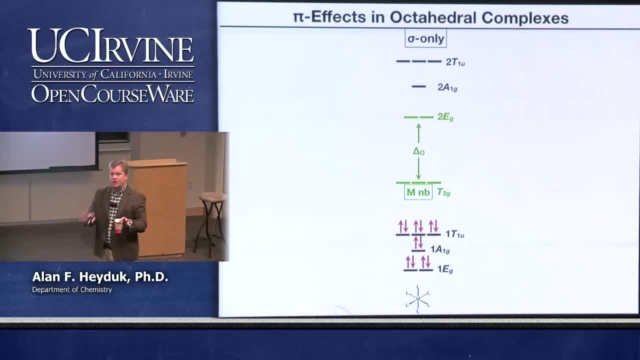 This middle case that I have is what we call the sigma only case. No pi bonding. This would be the case if you have six ammonia ligands Or six methyl ligands. No pi bonding. The only thing we're going to do is we're going to do this. 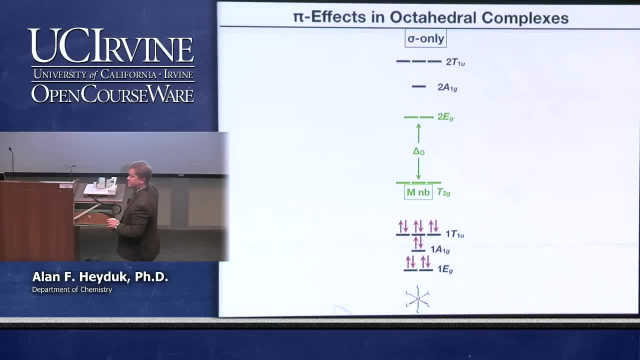 The only thing holding the ligands on are these six Lewis acid-Lewis-base interactions. In that case we know T2G is non-bonding And the separation to the EG is delta O. Okay, So now we can consider what happens. 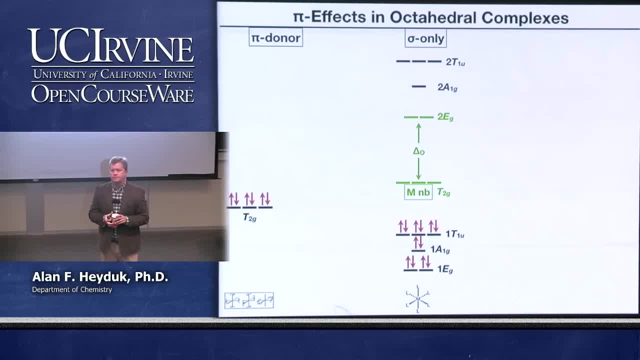 if we have pi donor ligands. These are halides, amides, oxo's heteroatoms, electronegative atoms with lone pairs of electrons in pi symmetry orbitals. There's only three symmetry adapted linear combinations that we need to worry about. 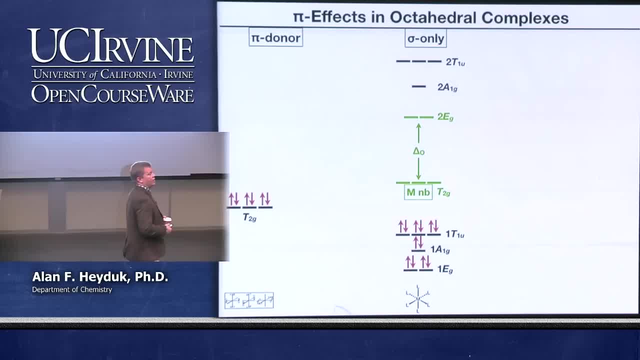 And we'll assume that all of them are populated. Now, if These are chlorides or bromides or oxo's, Those are electronegative elements, right? Those pairs of electrons are going to be lower in energy than the metal d orbitals. 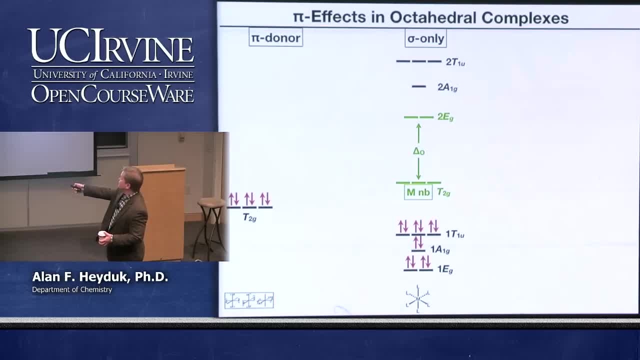 Right, And so we put them down here Below the non-bonding T2G orbitals of the metal. We know that when we have an orbital combination on the ligand set and an orbital combination on the metal that are of the same symmetry, we can make a bonding. 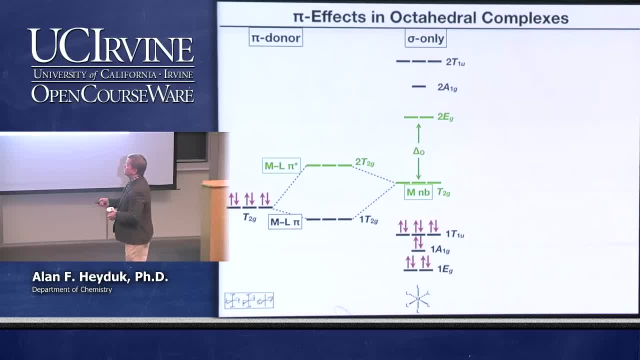 and an anti-bonding combination. So in this case, because the ligand lone pairs are lower in energy than the metal orbitals, the metal T2G, we can say that the ligand lone pairs are stabilized to make the metal ligand pi bond. 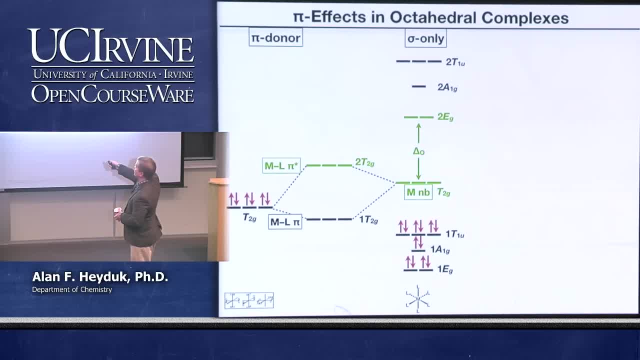 The metal orbitals. The metal T2G orbitals get destabilized to make the metal ligand pi, star. Those six electrons that were lone pairs on the ligands of course go into the pi bonding orbitals. Everything else from the diagram just gets transferred over. 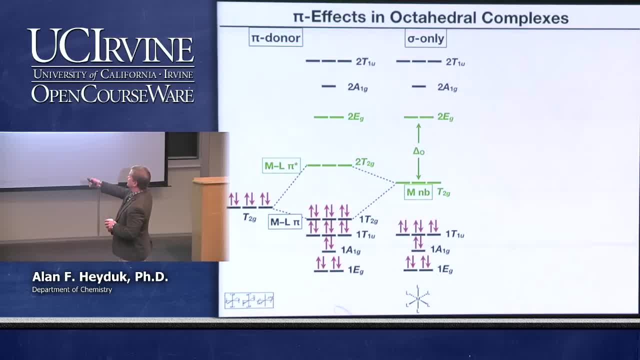 to a first approximation. Nothing happens to the sigma orbitals, Nothing happens to the EG orbital, Nothing happens to those four orbitals representing the metal S and the metal P orbitals. All that changes is we push up the T2G orbitals on the metal. 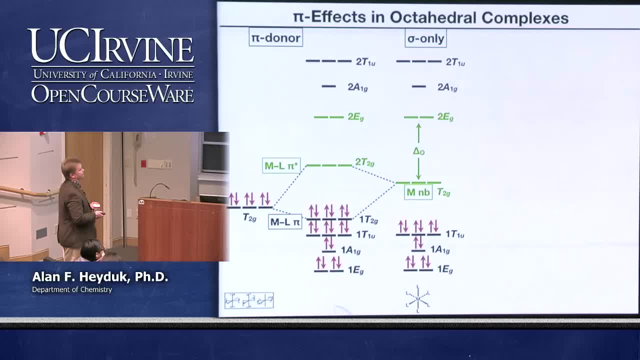 And we stabilize a few lone pairs on the ligand. So now the metal T2G is pi star instead of non-bonding, An important point here. If you look at these pictures, you look at the corresponding pictures that were on the last slide that describe these pi interactions. 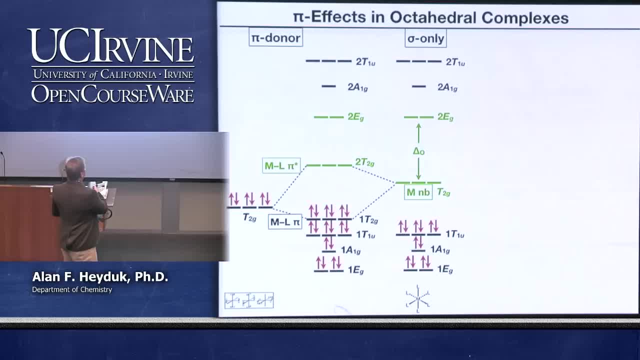 we're only stabilizing. we're only making three metal ligand pi bonds, But they're spread out over all six positions. Okay, So you don't really get double bonds between the metal and all six ligands. You can think of it as each metal ligand bond is now one. 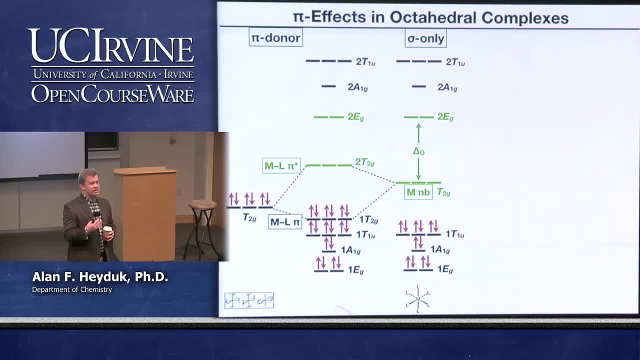 and a half. Okay, Because again you have three bonds, three pi bonds, spread out over six different ligands. We also can see why low D electron counts are favored here. Again, these orbitals in green are the metal D orbitals. 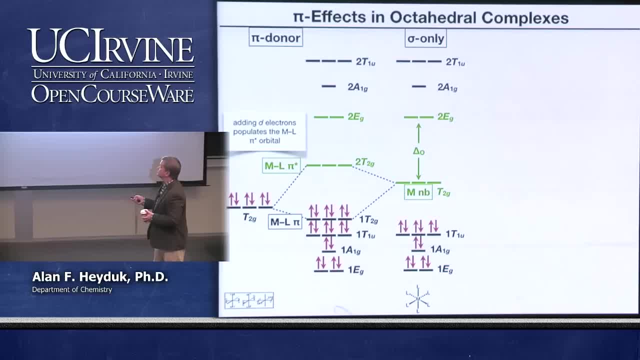 If we add three electrons, they're going to be non-bonding. Again, these orbitals are going to be non-bonding. Well, that means we put three electrons into these pi star orbitals. When you populate a pi star orbital, you destroy the pi bond. 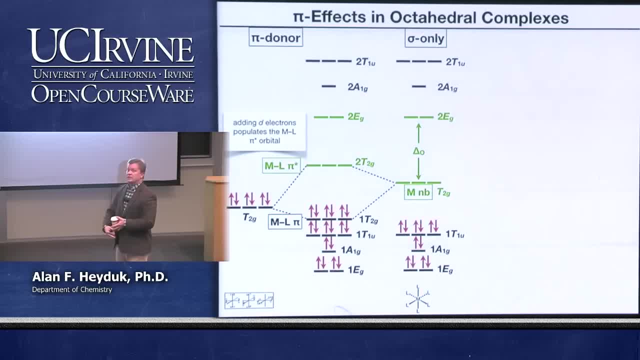 If we were to put six electrons in here, we'd completely destroy the metal ligand. pi bonding The sigma bonds would still be okay, We'd still have sigma bonds, but we would have no pi interactions. So how are pi acceptor ligands different? It turns out, the symmetry of the orbitals on the ligand are exactly the same: T2G. The difference is they're typically something like a pi star orbital on the ligand, So for instance, a CO pi anti-bonding orbital. 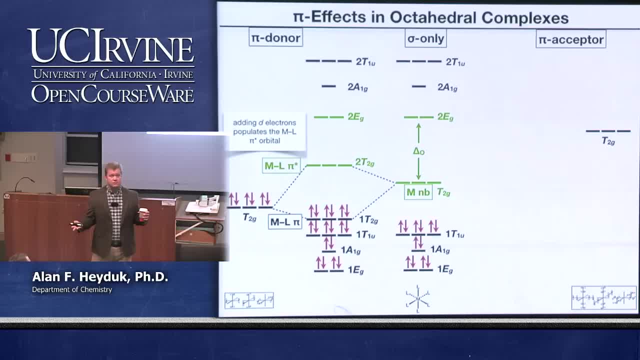 We know anti-bonding orbitals are typically high in energy, So now this T2G set on the ligand ends up being higher in energy than the metal non-bonding Ds. We can still make a bonding combination and an anti-bonding combination. 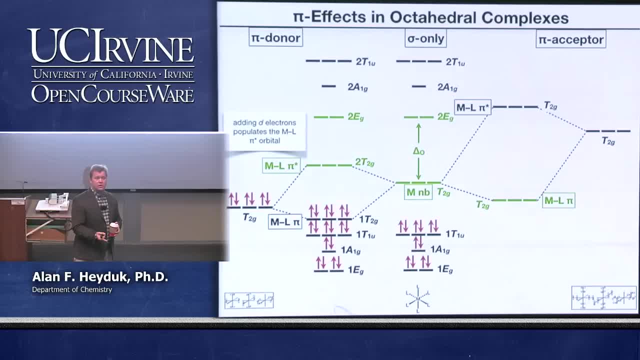 But in this case, look at how things were color coded. The T2G orbitals on the metal are lower in energy. They're not the same. They're not the same. They're not the same energy than the T2G orbitals on the ligand. 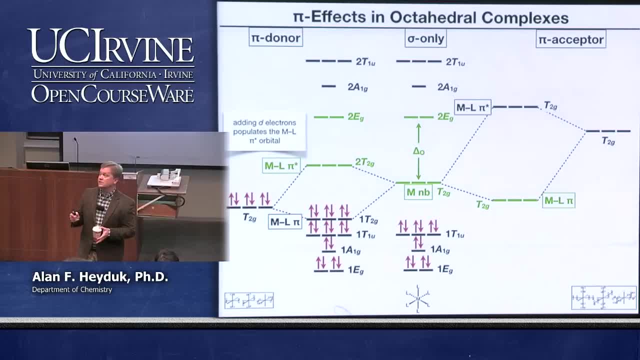 So the bonding orbital is localized on the metal And the anti-bonding orbital is localized on the ligand. It's the exact opposite case of the pi donor ligand. Now the metal D orbitals are metal ligand, pi bonding, And the ligand orbitals, the CO pi star, is anti-bonding. 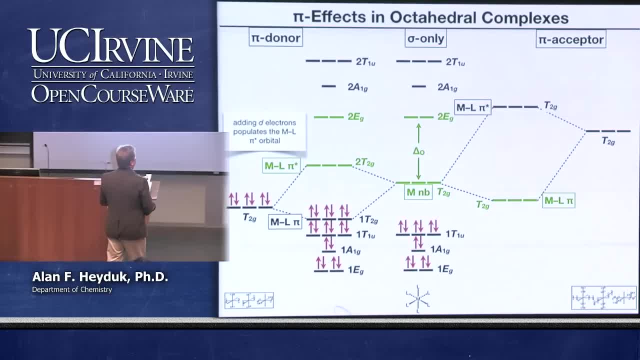 Primarily The rest of the diagram. just like we saw before, we can carry across to a first approximation. The sigma orbitals don't really change. The EG orbitals, DZ squared and DX squared, minus Y squared, don't change. 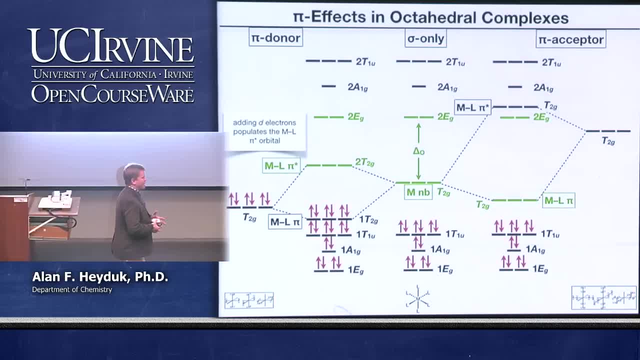 The metal S, the metal P still remained metal ligand, sigma star. We can put electrons in here If we add D electrons. well, that's actually what makes the bond. If we have no D electrons, then we have no pi bond. 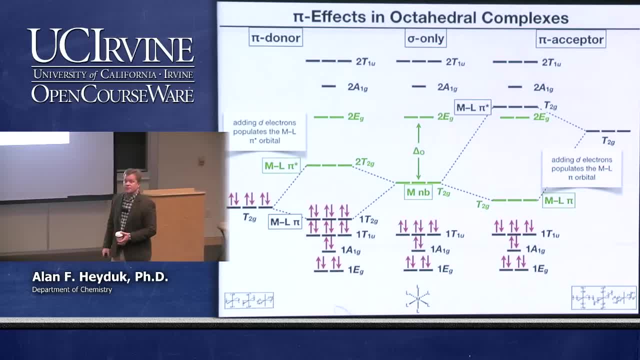 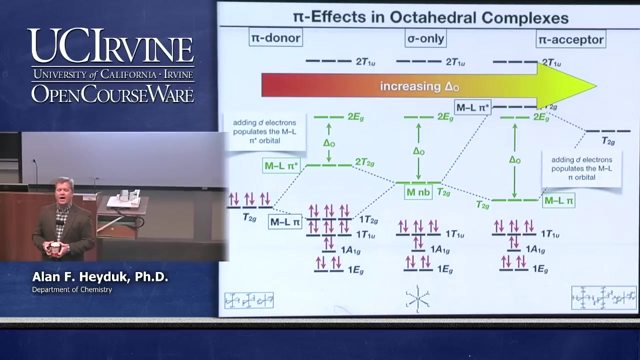 But you can see, ideally we'd have a D6 low spin electron configuration, Because that would fill up this metal ligand, pi bonding orbital manifold. And so what's the big difference? When we have pi donor ligands we end up with a relatively small value for delta O. 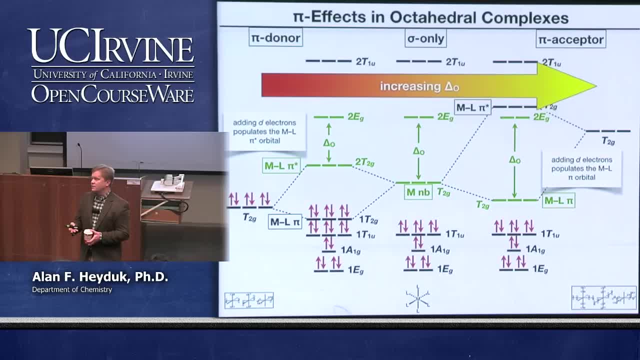 The splitting between the T2G orbitals on the metal and the EG orbitals on the metal is typically small When we have pi acceptor ligands. remember, T2G got stabilized, So now delta O is really large. It's large because T2G was dropped in energy to make these pi bonds. 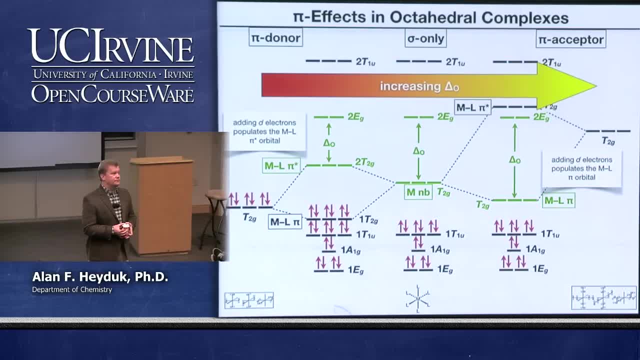 For the sigma only case. it's right in the middle. Now, why do you think this is important? It plays right into the idea of high spin versus low spin. The magnitude of delta O is critical to whether our complex is going to be high spin or low spin. 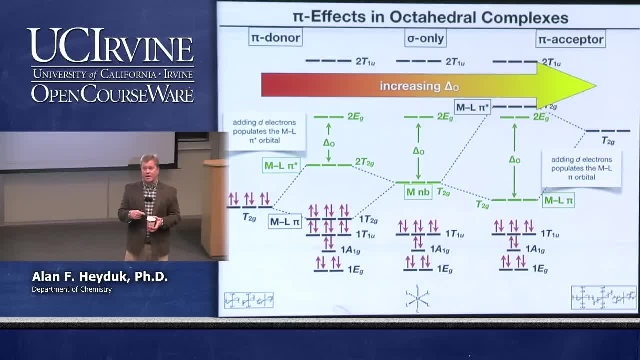 When delta O is smaller than the pairing energy, you're going to put an electron up here before you pair it up down there. When delta O is larger than the pairing energy energy, well then you're going to put two electrons down here before you populate EG. 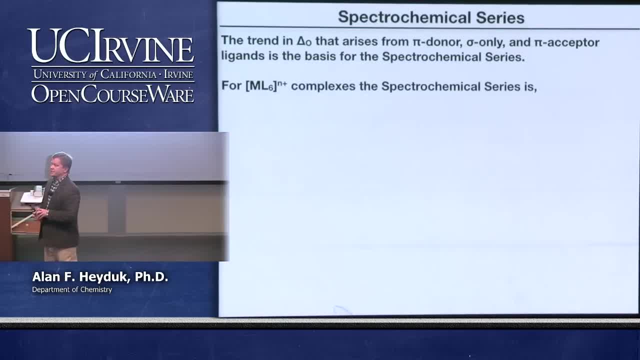 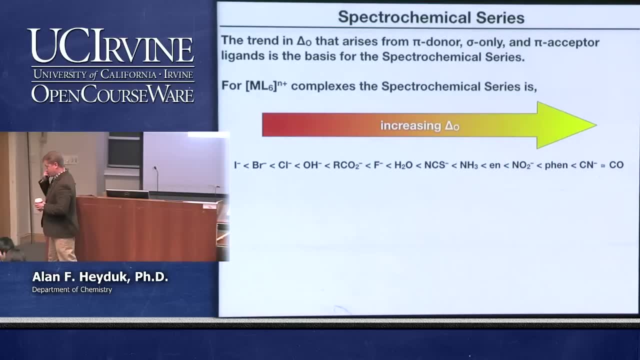 That trend is what we call the spectrochemical series. So in the spectrochemical series you'll see various versions of this, some with different ligands included. I just picked a few common ligands so that they all fit on a slide. You can imagine if we had every known ligand. it would go off the slide and be really hard. 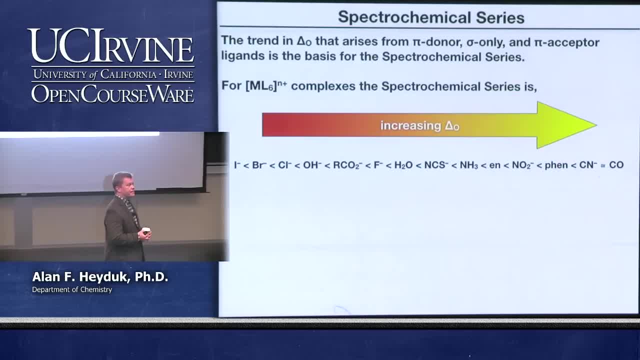 to read and basically useless. But we can look at this series. we can say, oh, over here on the left, where we have small delta O values, we have pi donor ligands, Ligands with lone pairs of electrons that can donate to the metal. 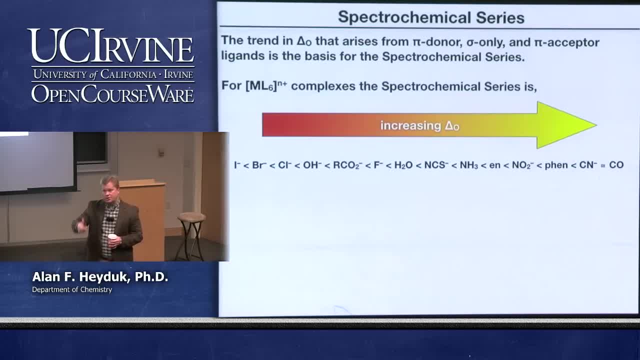 That donation of the extra lone pairs is going to push up T2G and make delta O small. In the middle we have water, ammonia, thiocyanate. Those pretty much are the sigma, only ligands. They have no pi interaction. 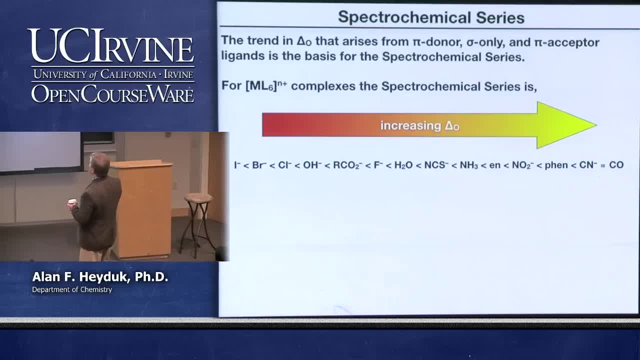 They have no interaction with the metal whatsoever. Over on the right side, carbon monoxide, to some extent, cyanide, phenanthroline- those are pi acceptor ligands. They have empty pi star orbitals that can accept electron density back from the metal. 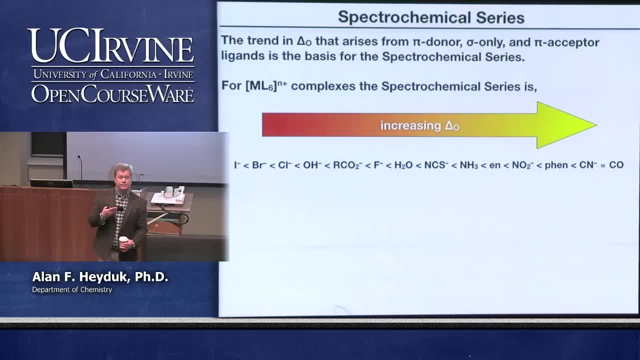 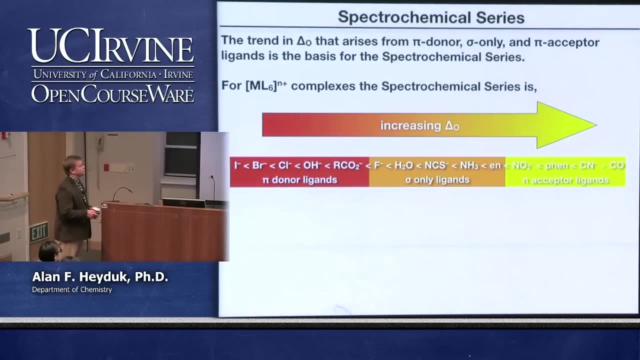 and in doing so they stabilize T2G. When they stabilize the metal T2G orbitals, delta O gets bigger. Generally speaking, when we're talking about octahedral metal complexes of the first row of the transition metals- if you see a ligand here in the red- 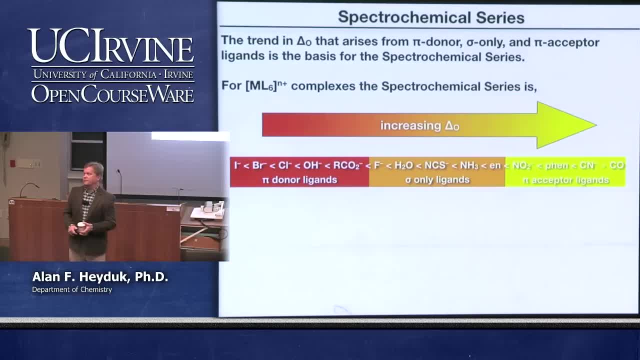 If it's a pi donor ligand, I guarantee you it's going to be high-spin. If you see ligands here in the orange with sigma, OH could go either way. If you see ligands over here in the yellow- the pi acceptors- it's almost always going. 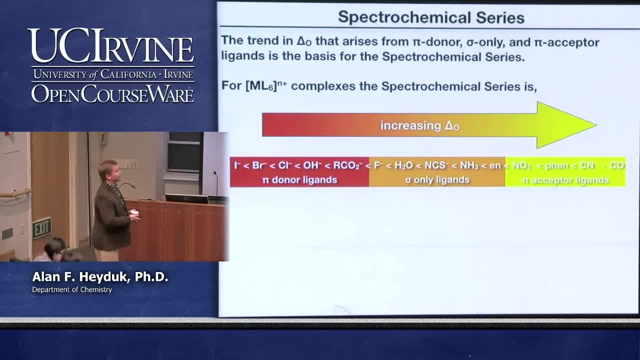 to be low spin because these pi acceptor ligands give large delta SOs, much larger than the octahedral orpex use. All right, And what are they really? They can be going anywhere in the next 20 to 25 years if we give them value of pi now. 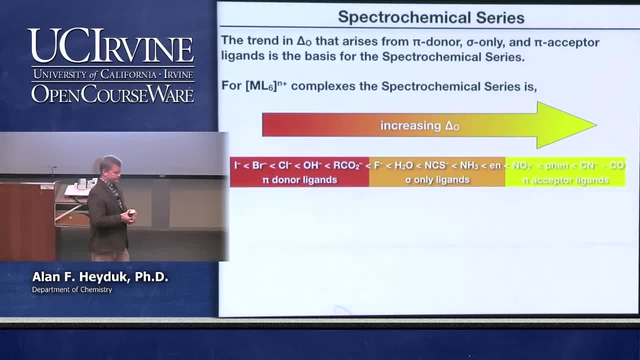 larger than the pairing energy. Now, we're talking about this kind of at a very kind of at an entry level, okay, But you can also think about it a little bit more deeply. Well, what's pairing energy, Dominated by the repulsive interaction of putting two charges in a small space? 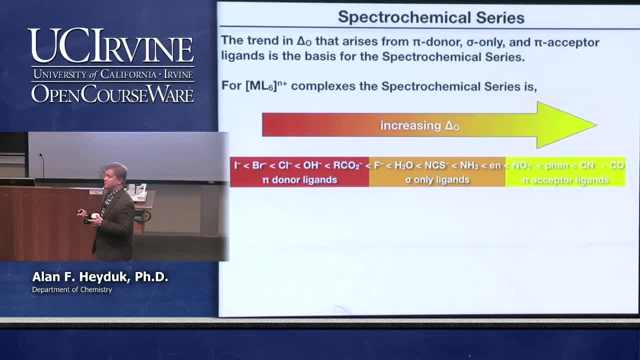 So if you have smaller orbitals, the pairing energy is going to be larger, And so if you have an orbital, a d-orbital, that's now been delocalized over a pi acceptor ligand, that in effect makes the d-orbital bigger. 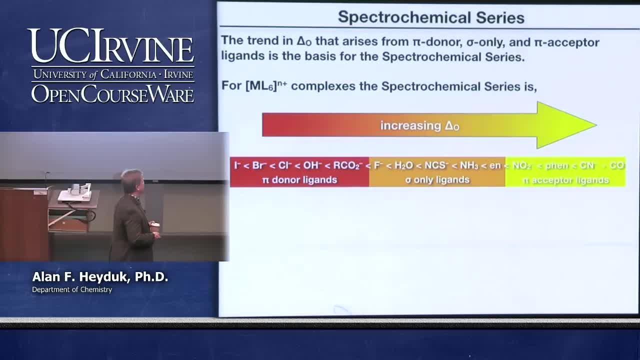 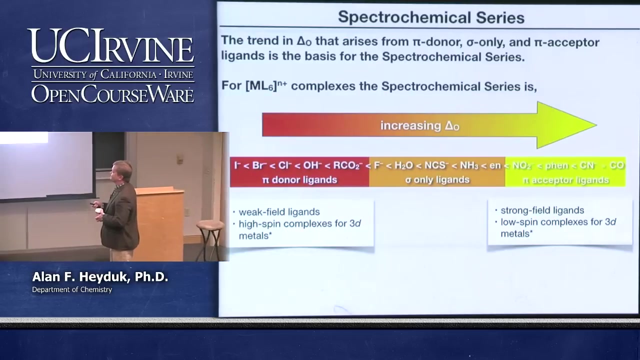 Okay, It also helps lower the pairing energy, But these are just things that I want you to think about, Because at this point in your careers, you know there's always more to the story than you get in class. Don't you love the asterisk? 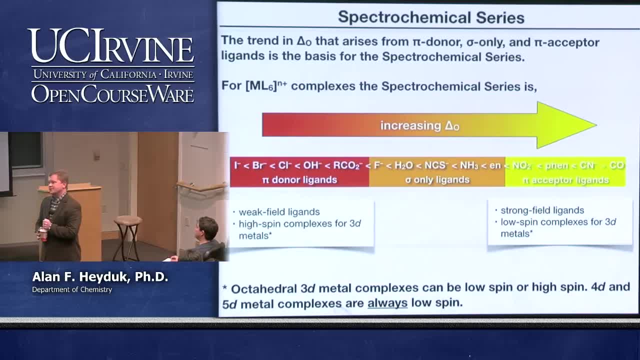 So again I want to reemphasize Octahedral metals or octahedral complexes of the 3-D metals can be high spin or low spin. Octahedral complexes of the 4-D and 5-D metals are always low spin. 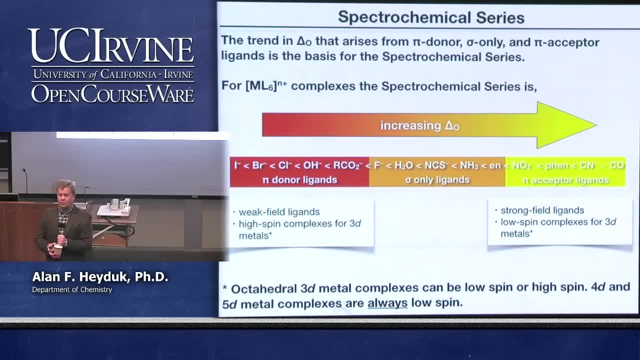 Delta O for a 4-D or a 5-D metal is always large, Much larger than the pairing energy. That again there's two reasons. Okay, The first reason is the 4-D and 5-D metals make stronger metal ligand sigma bonds. 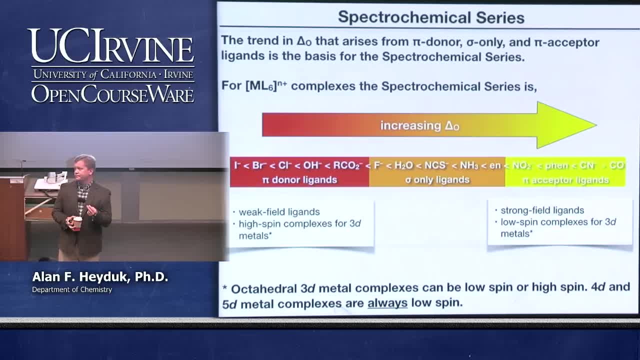 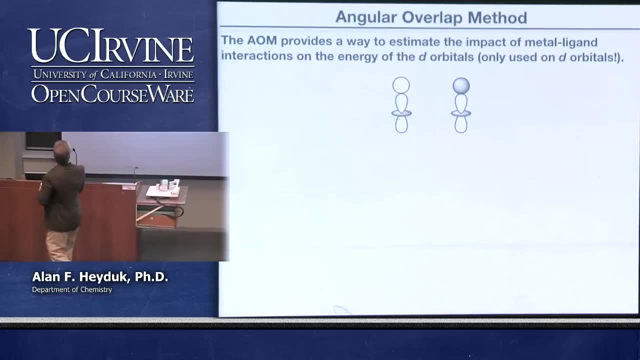 The second reason: duh, 4-D and 5-D orbitals are bigger. A bigger orbital means a smaller pairing energy. Okay, So one of the most difficult things to do, Okay, One of the most difficult things when we're constructing these ligand field diagrams, or 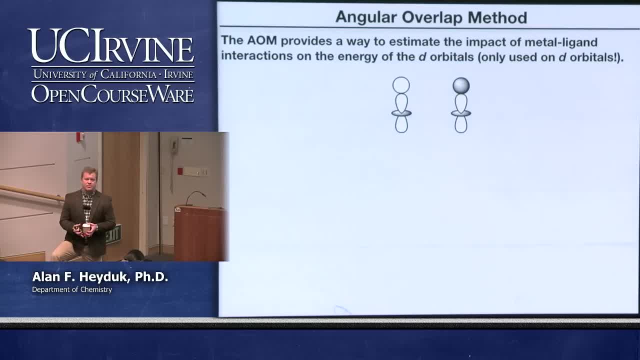 these molecular orbital diagrams, especially when you're starting out, is figuring out how far up to push something or how far down to stabilize something, And trust me, it gets better with experience. I hate to say it, but not much Okay. 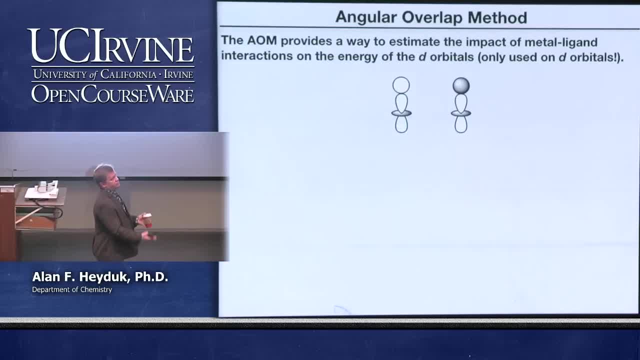 You're always saying, well, did I make that too anti-bonding or too okay? So this angular overlap method was developed to help answer that question, To kind of give you numbers that you can calculate, to make it a little bit easier to figure out. 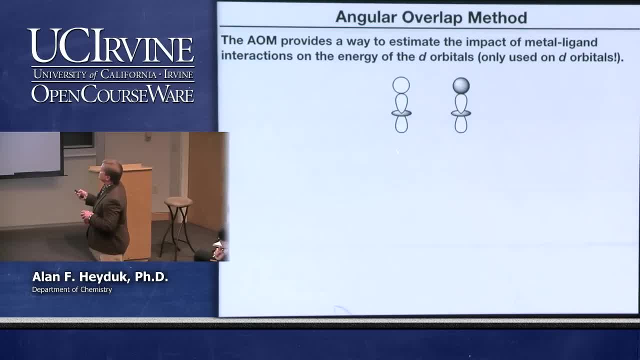 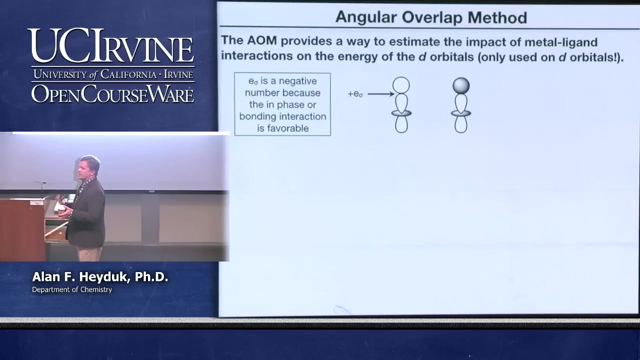 well, did I push that up far enough or not? The angular overlap model is based on this sigma interaction: A single pair of electrons being or interacting Or interacted with a DZ squared orbital on the metal. When that interaction is in phase, the value is assigned E sigma. 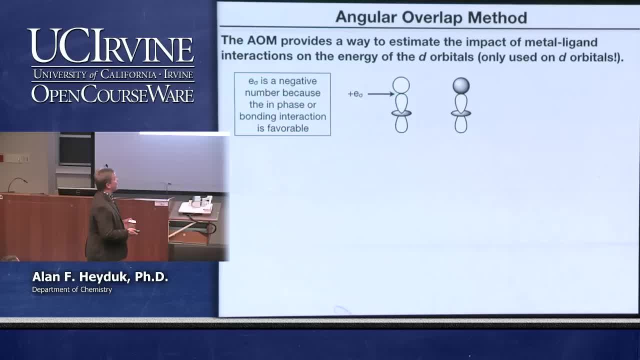 Okay, It's a stabilizing interaction. When it's out of phase, we say that it's minus E sigma, Just to confuse you, right? Because E sigma is actually going to be a negative number. So If you keep a positive negative number, then that's going to be down. 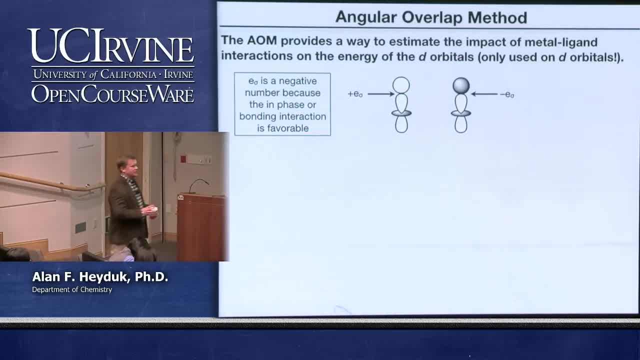 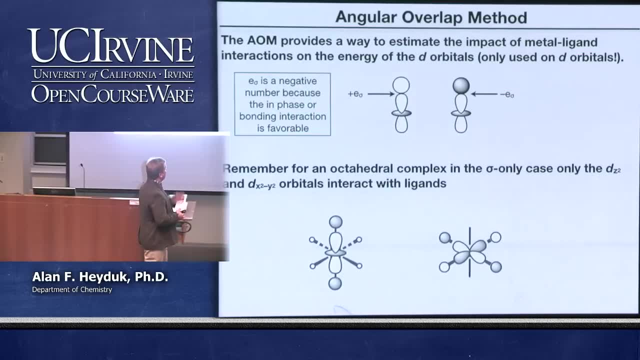 And if you take a negative of a negative number, that's going to be up. Just remember our energy convention in science is always great, Okay, And so the way that this works, we know for an octahedral complex that we have two D orbitals. 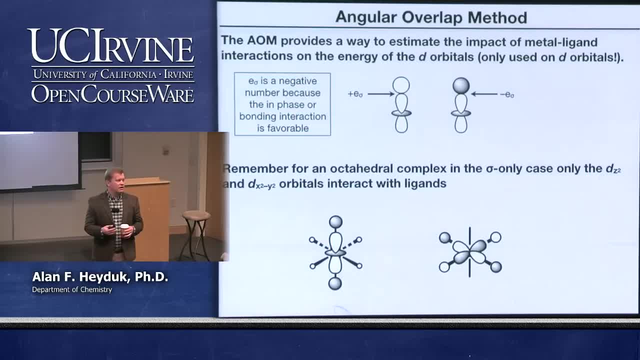 that are metal ligand, anti-bonding DZ squared And DX squared minus Y squared. We know that they're degenerate Exactly the same energy by symmetry. They have to have identical energies, And so the way that we, the way that this is treated, is we say okay, again, that's. 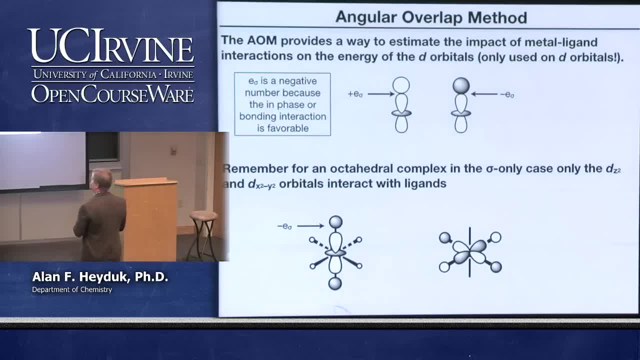 a minus E sigma because it's an out of phase combination. That's a minus E sigma because it's an out of phase combination. That's a minus one quarter E sigma because it's an out of phase combination. Well, why is it so much smaller? 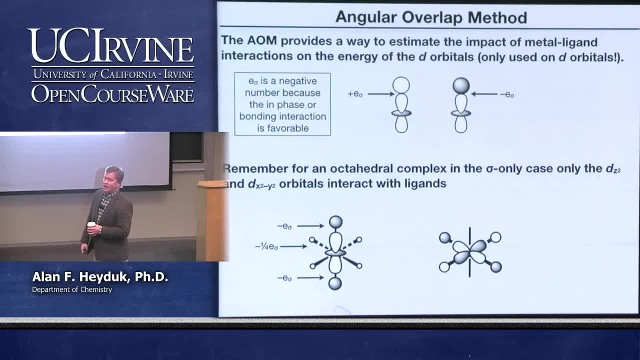 Well, first because that's a donut on DZ squared And also because, remember, when we calculated the symmetry adapted linear combination of orbitals on the ligand that has a much smaller coefficient. It's much smaller in size than that, So that interaction is going to be weaker. 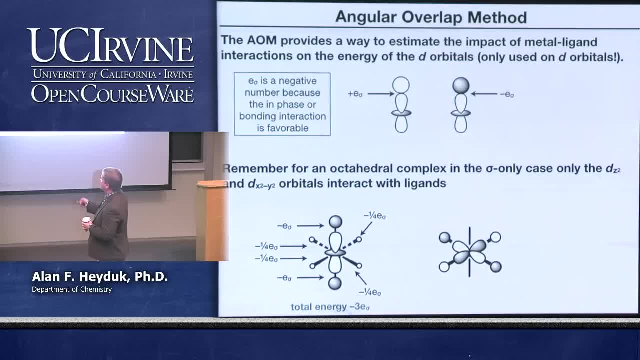 Okay, Now if you tally it all up, we calculate that the total energy of the metal DZ squared- So this is the metal ligand anti-bonding orbital- is going to be minus three E sigma. So our challenge with the angular overlap model is to figure out the energy of that. 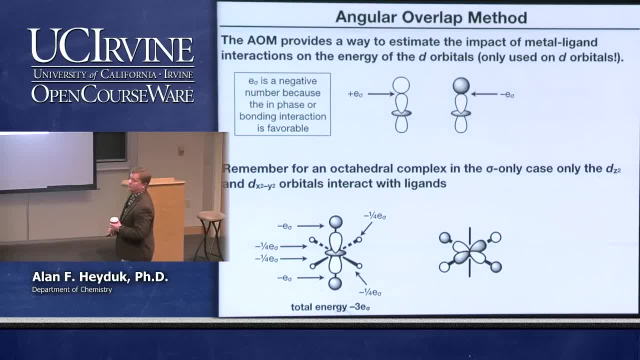 Well, we know it has to be my total minus three E sigma, And so the way that we get it is to say that each one of them has to be minus three E sigma. Okay, One of those interactions is minus three quarters E sigma to give us again a total energy. 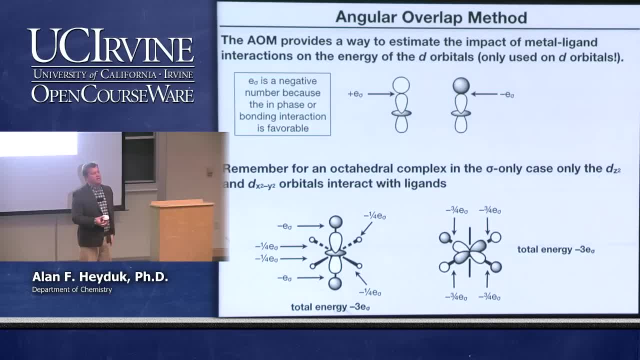 of minus three E sigma. Now again you're saying: well, wait a second. Why is this one minus E sigma and this one minus three quarters E sigma? The DZ squared orbital has a stronger projection along the Z axis than the X squared minus. 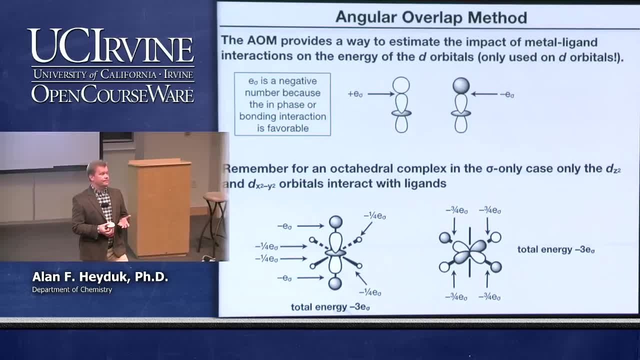 Y squared orbital has. Okay, So the DZ squared orbital has a stronger projection along the X or the Y axis. Okay, Similarly, the coefficient on that ligand orbital is larger than the coefficient on that orbital, So it just is a stronger interaction along that Z axis. 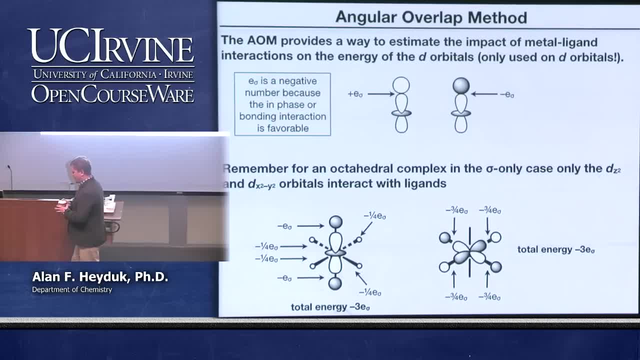 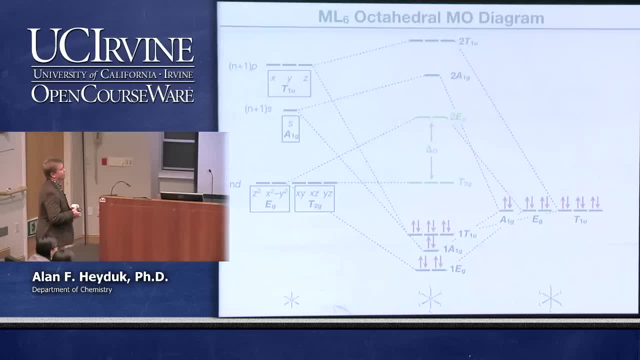 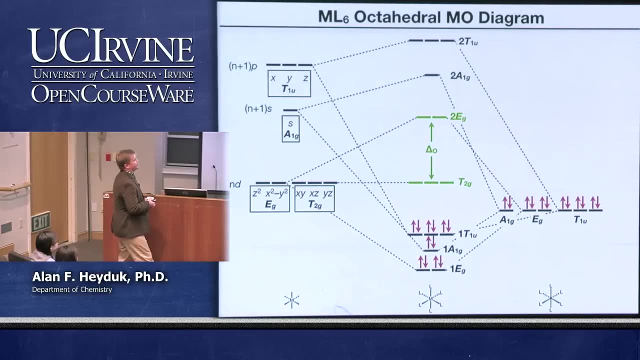 But through some remarkable reverse engineering, the two orbitals come out to be the exact same energy. Okay, So now, if we come back to our sigma-only octahedral diagram, remember we said this: splitting between T2G and EG was approximately delta O. In the sigma-only case, these are: 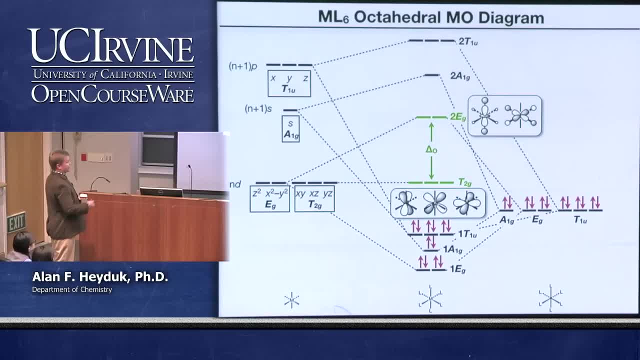 nonbonding. There's your two EG orbitals that we just looked at. We can say that that energy delta O is approximately three E sigma. Okay, So it's a different way to count up the separation between the T2G orbitals and. 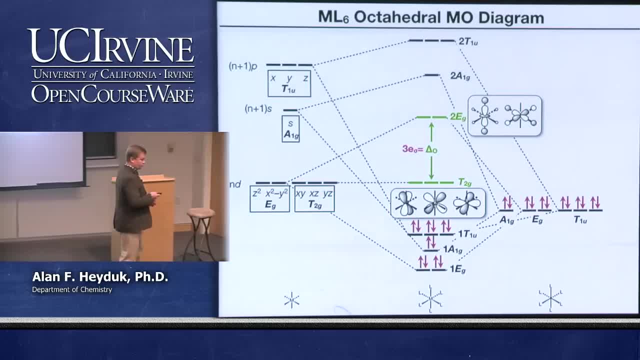 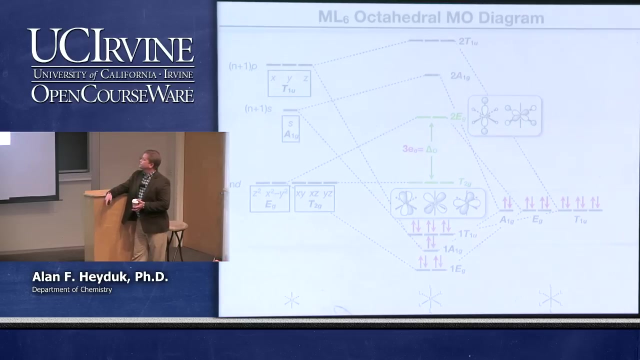 the EG orbitals. You'll see in your textbook that you can also use this angular overlap model to estimate the interaction between the metal and the ligands for the pi bonding as well. It brings in another variable, E pi. So how do we use this angular overlap model? 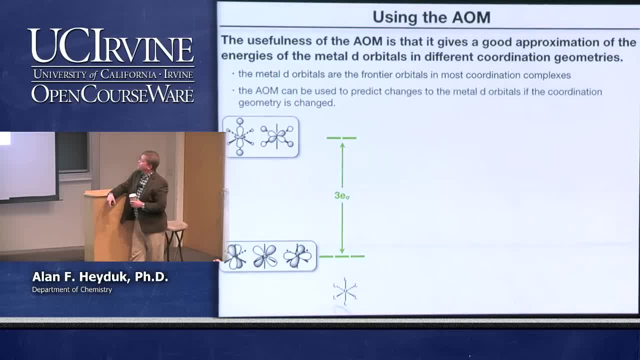 Just real briefly. we'll pick up here on Wednesday. If this is our frontier d- orbital splitting for a sigma-only octahedron, we can do the thought experiment. What would happen if we went from an octahedral complex to a square pyramidal complex? 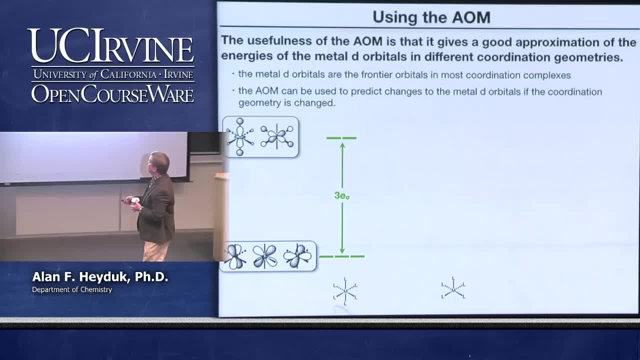 We remove one ligand. In that case T2G does not move, but and neither does X squared minus Y squared. but DZ squared now comes down. So it gives us the ability to make a quick estimate of how much to stabilize the DZ squared orbital. 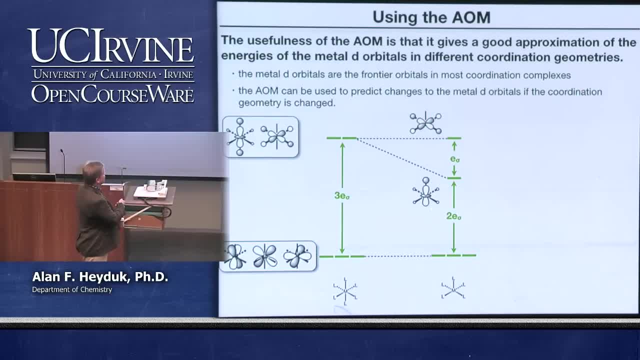 because we removed one antibonding interaction. Same thing. we can ask what happens if we remove that other axial ligand. Well, now, what we've done is derived the d orbital splitting diagram for a square planar complex, right? So if you know what an octahedron looks like, 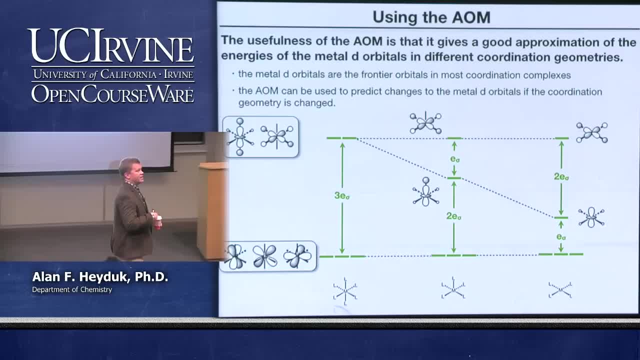 and you know the approximate angular overlap energies. you can immediately predict what square planar is going to look like by just removing one and then a second axial interaction. And so that's what we're going to do, And so what you find out for square planar complexes. 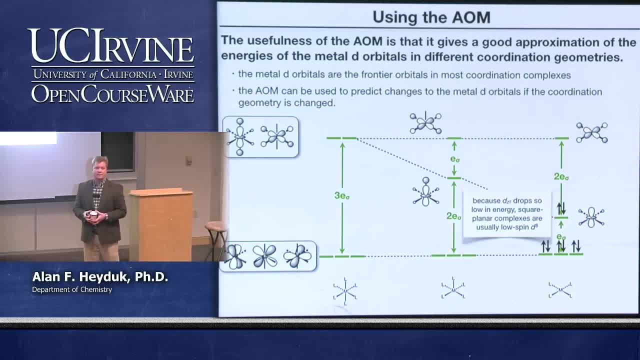 they're usually low spin, they're usually D8, and if you remember, back a couple of lectures ago, I said, oh, any time I see a square planar platinum complex, I know that it's platinum 2, because platinum 2 is D8.. 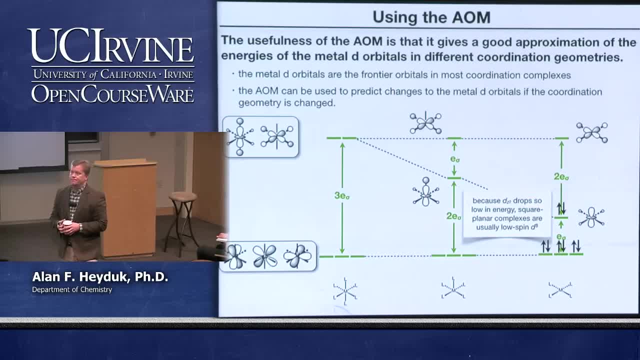 And that's how you stabilize a square planar geometry. So we'll pick up here on Wednesday. Have a great rest of your morning and a great afternoon. 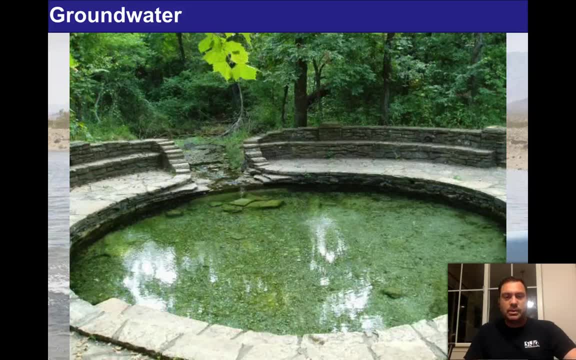 Hey everybody and welcome back. Today we're going to be covering some new information to follow on to our last lecture on surface water. We're going to be talking about groundwater. Surface water is fascinating stuff. You know that last lecture had a lot of information in it. It covers a lot of details about how rivers work and transport sediment and all the different features associated with rivers. 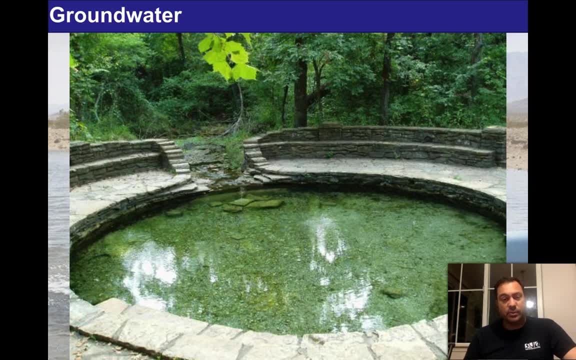 Well, groundwater has its own features, and some of those are really really interesting and important, And so we're going to jump right in. So this whole lecture is going to be about groundwater and its importance to human beings. So here, we see a pool of water here, and we might be asking ourselves: what's the source of the water? Are they bringing it in?